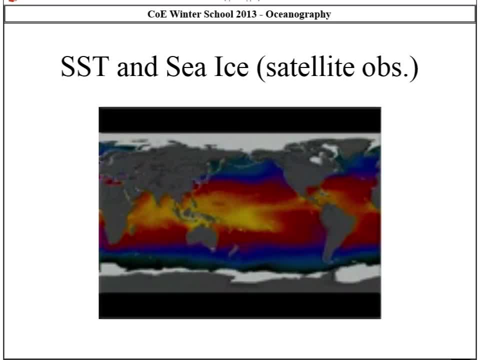 Okay, tell me, what do you see? Let's play a little basic pattern recognition. What do you see here? What do you? what captures your mind? Reptile currents, Reptile currents. You can see some things going on along here, eh. 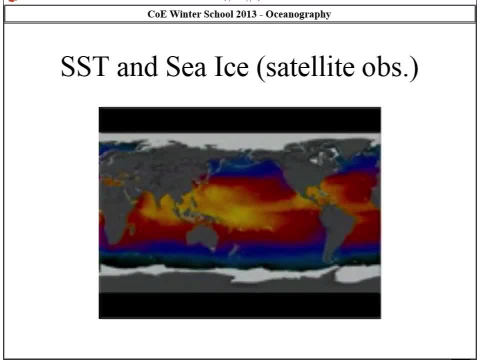 What is the basic pattern structure of the temperature of the surface of the ocean? Zonal, Zonal, yeah. So what do you mean by that? You see the temperature, You see the temperature. You see the temperature. It's a cold in the east-west climate. 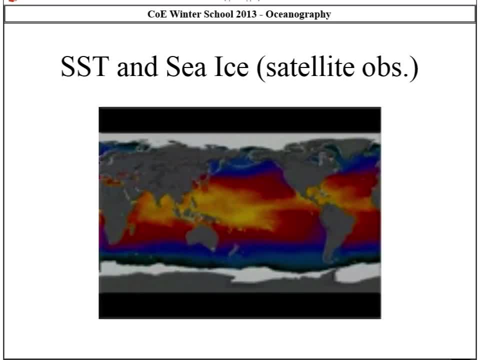 East-west direction. Yeah, Okay, let's make it even simpler. Where is the water warm? The orange is the warm stuff, the blue is the cold stuff. Low Warm in the middle, Cold at the poles. You see other patterns there. 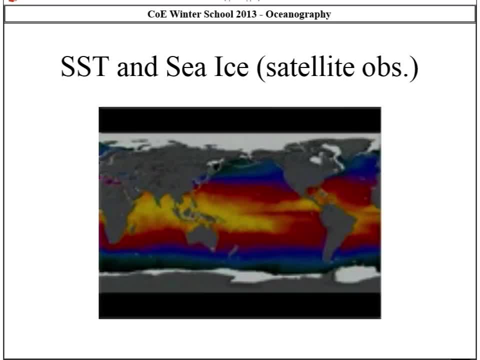 Yeah, Warm in the middle, Another one. I like Warm on the west relative to the east. Good, Anything else You notice in this little picture? Sea ice is moving a lot with the seasons. Yeah, You see a lot of squiggles in there too, right, Lots and lots of squiggles going on. 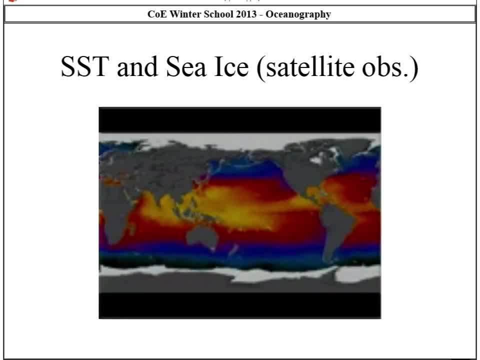 Okay, let's imagine a sphere covered in water, A rotating sphere covered in water. In my mind, there's no reason why that water should be moving. So question number one: why is the water moving? Why does the ocean move? 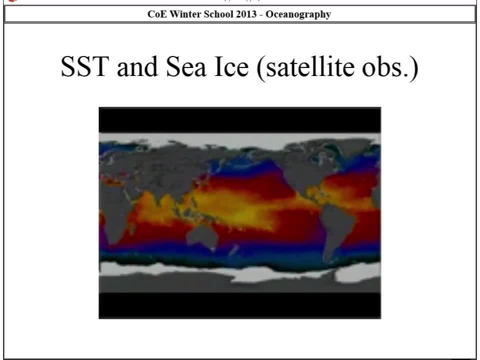 Wind stress. Yeah, there's forces on it. Okay, Why does the wind move? Differences in temperature. I can see that we're all on the same page. The ocean moves and the atmosphere moves around, largely because of the temperature. The ocean moves and the atmosphere moves around largely because of the temperature. 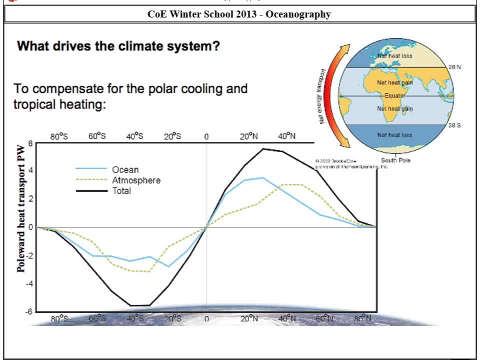 And the temperature moves and the atmosphere moves around, largely because of differential heating. Okay, I think we're mostly aware that it's warmer in the tropics than it is at the poles, So to a large extent you can think of the climate system as a heat engine. 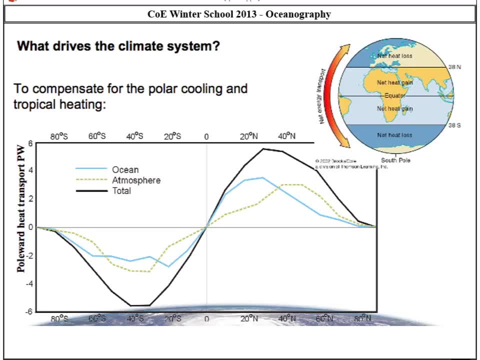 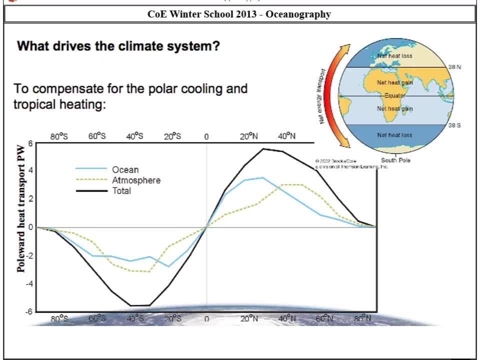 source of differential heat. Can we read some other ones? Seasonal cycle, It's a great one. Other ones: Land versus ocean, Land versus ocean, People in the back. What's going on back there? What else is another source of differential heat? 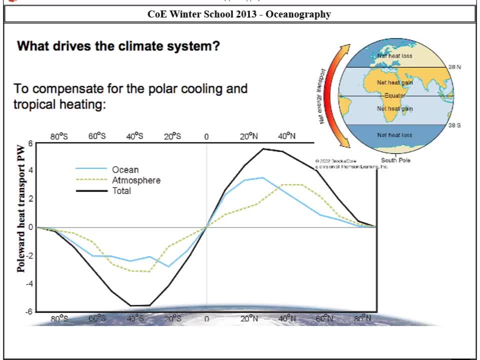 I heard I'm supposed to run around in the room to wake you up. Changes in the Earth's orbit around the sun, perhaps, And the way I tend to think of the ocean or the atmosphere is I kind of think of it. I used to work my first job. 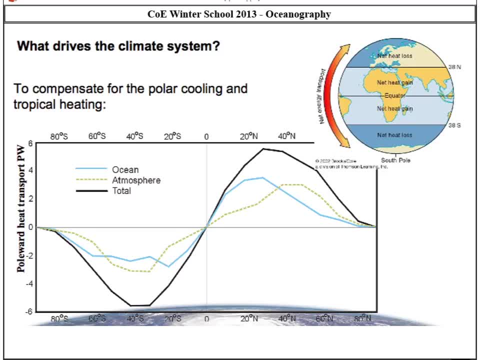 ever was at the trampoline center, Jumped the gym in the trampoline center And I kind of think of the climate system, all these differential heatings, as different sized kids jumping on the same trampoline, Or another way to think of it is. 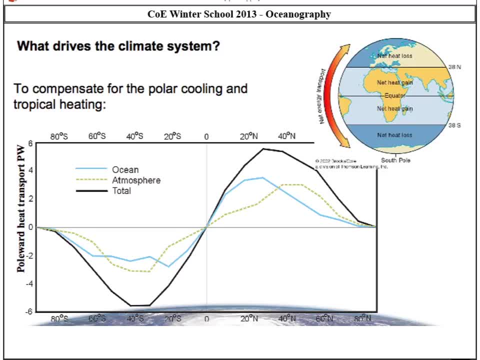 the planet Earth is like the skin of the drum with different beats on it. So the day and night cycle you can imagine is, you know, the young kid who's got lots of energy jumping- doesn't weigh very much Changes in the Earth's orbit. 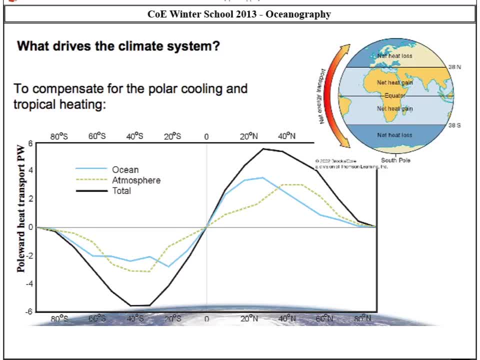 around the sun are kind of like, you know, a retired sumo wrestler Just breathing. And when you have a lot of people jumping on a trampoline- what sometimes happens- You get the super bounce. sometimes, right, Boom, Go away right. 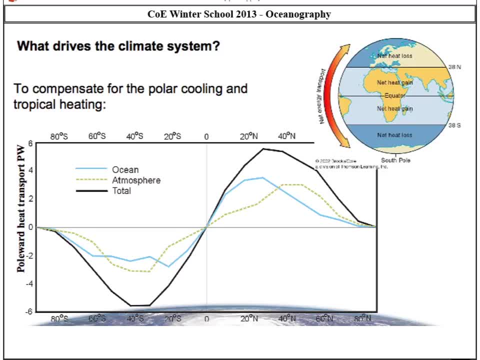 And other times you sort of go whoop And it doesn't happen. So I kind of think you know, all these different differential heatings are sort of bouncing around the system and they can interact with each other, making all sorts of interesting things. 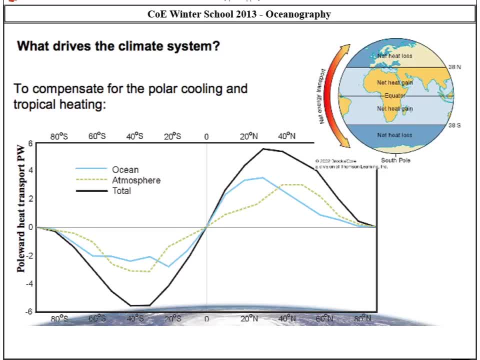 Right, oh yes, okay, Let's imagine there's no way I'm going to be throwing myself. that's it. What do we know? what do we know? We have the ocean south north. this is going down in depth. 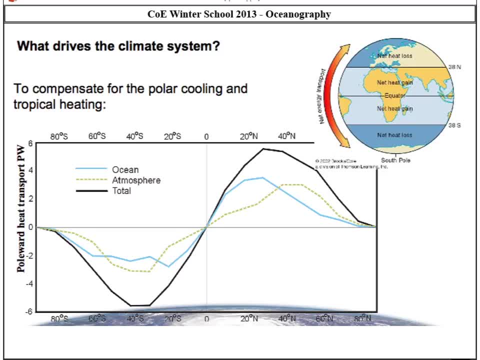 This is the ocean And we know that it's warm here at the top and it's cold here, cold here. Someone come up here and draw what type of ocean circulation they would expect under this kind of scenario. All I'm telling you is that we know now it's warm here and cold here at the surface. 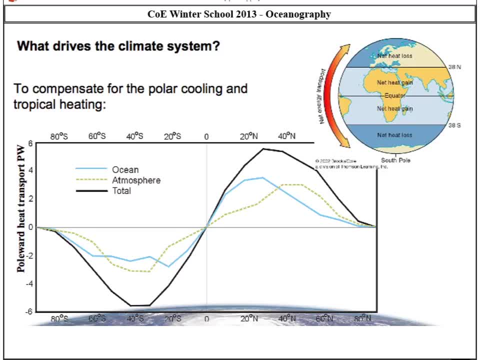 What type of an ocean? what do you think we're having? We have, like a big bathtub. There you go. Come on, No one said this was going to be easy. Well, I think you might have. Don't be shy, it's okay. 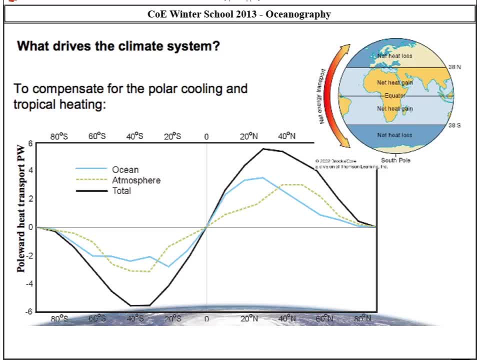 I actually think this is a really hard question. so Wouldn't you expect to just get an overturning switch? Oh yeah, And you know what? That's what they thought. We were wrong, right, Well, you know what? it's kind of surprising. 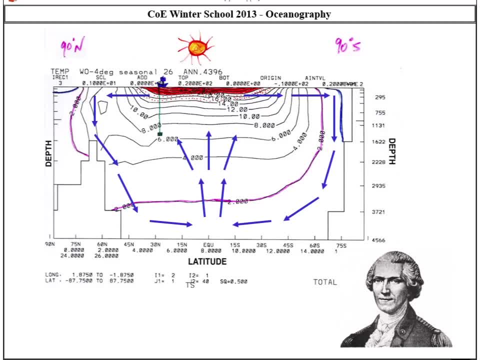 Because you can easily, As you can easily imagine, you know, in the Flat Earth Society you kind of think: well, maybe this water just gets warm all the way down to the bottom. And that's actually what they thought Until the first deep ocean temperature measurement was done in 1751, not that long ago. 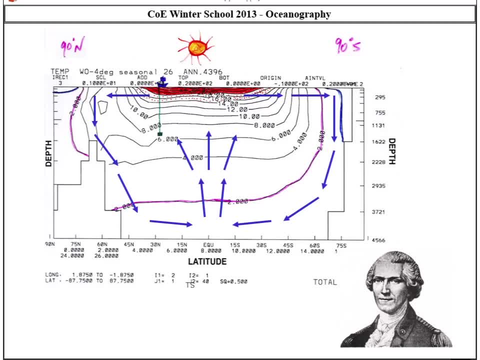 by Captain Henry Ellis When he had a fancy bucket in the tropics and he dropped it down and he got the water. How was he fucking fancy? He hadn't. I don't know the gory details of it, but it had like valves so that he could trap some water. Yeah, like little Yeah. so it wasn't going to get completely mixed as he brought it up. It wasn't just a normal bucket. Some famous English guy asked him to do this when he was out there. He brought it up and he was very excited to learn that it got extremely cold at the bottom of the tropics. 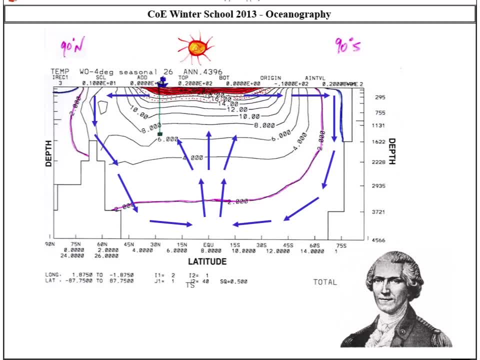 You know, down to three to five degrees Celsius down there. Why he was very excited about this is because he was He was a drunken slave trader And they used this to cool their wine and booze on the boat because they were in the tropics and they were just letting on. 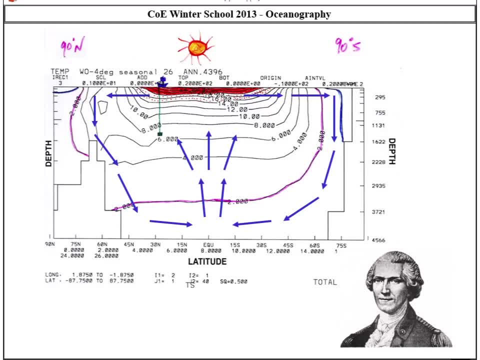 It's true. So to a large extent this is sort of the foundation of the global thermohaline circulation. So the great careers of people like Matthew England and all these other people were built on the discovery of a drunken slave trader in 1751.. 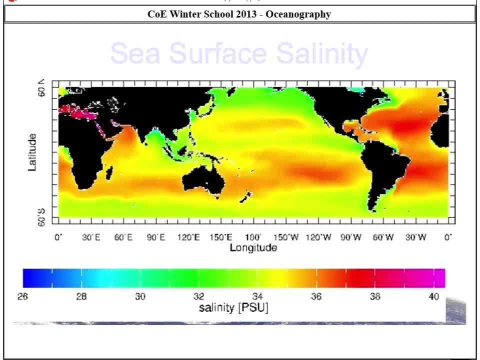 Okay, Onwards Salinity. This is a map of sea surface salinity around the planet. The red stuff is salty, The blue stuff is relatively fresh. Again, what do you see? Where are the pyramids? Yes, sir. 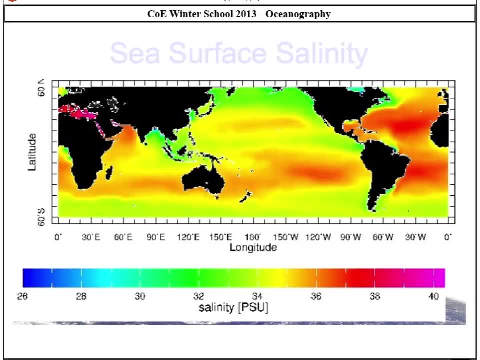 It seems to be a little bit saltier in the Mediterranean. Very salty in the Mediterranean, Yeah, True, What else do you see? Subtropics are saltier. Subtropics are saltier. These spots are salty, Yeah. 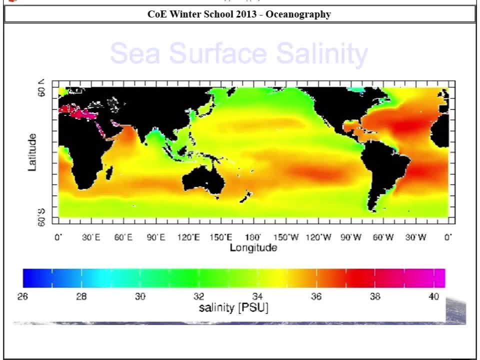 Anything else. I'm out by the flow of major rivers, like over by India or the sea. Yeah, Florence is a lot fresher. This is the Orinoco, the Amazon. I'm not very good with rivers- Congo, Yeah. 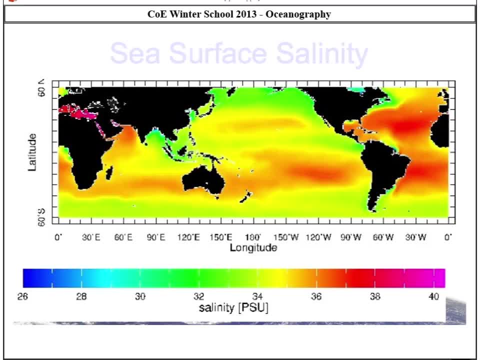 Rivers Fresh. What else do you see? The Atlantic is saltier than the Pacific. Okay, Now let's go a little bit into the why. Okay, First, why is the Atlantic saltier than the Pacific? Less circulation, I think, that's. 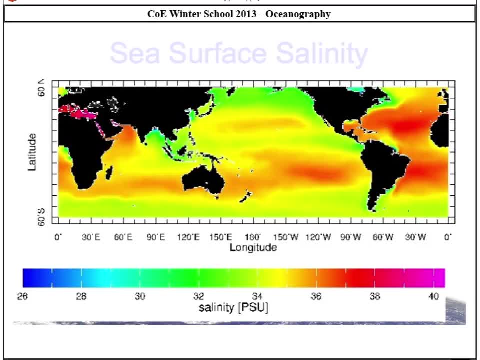 Well, that's circulation, where, Well you know, just imagine maybe like the giles or something, and then That's a good guess. Yeah, I don't think that's the answer. I'm not. Yeah, Okay, So what determines the salinity of the ocean? 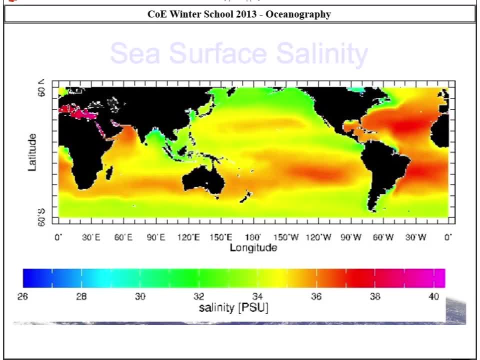 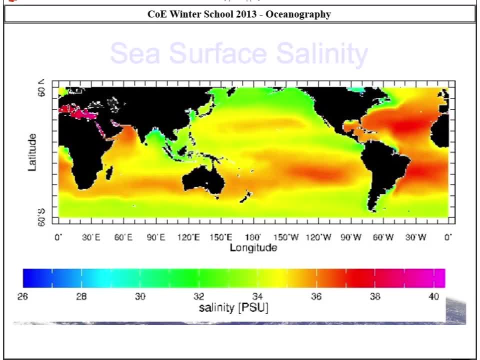 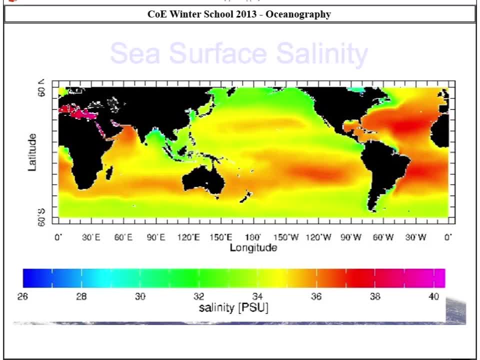 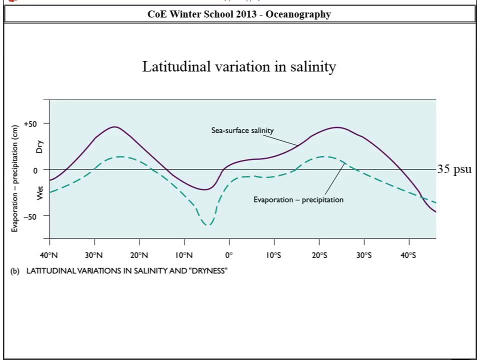 And so we take a zonal average of the salinity of the ocean. this is just going from 40 to 47. So in the tropics, certainly when you go to the poles, melting sea, ice production, sea ice, it's going to matter. 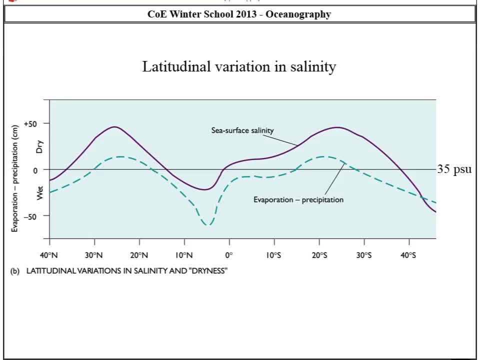 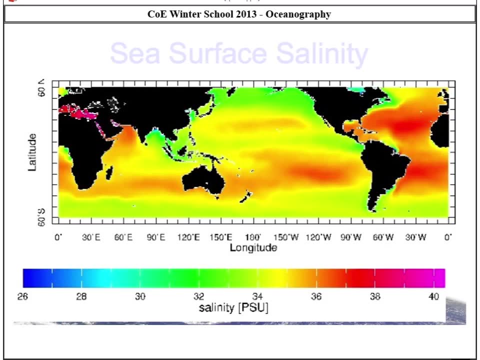 In the tropics, the sea surface salinity really pretty much follows evaporation minus precipitation. Okay, okay, so what we're seeing here is patterns of evaporation minus precipitation. we have really salty regions here, right around 30 north and 30 south. it is no coincidence. 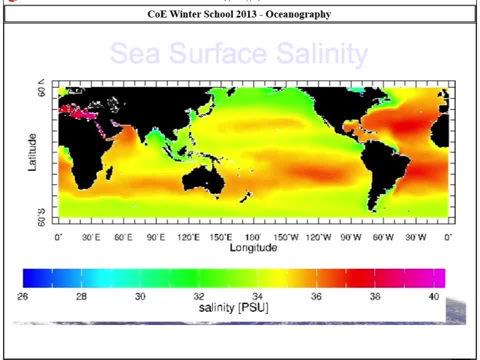 that this is at the same latitude of all of the world's major deserts. right, Australia? I don't really know what's going on here. it's pretty dry here. I haven't been there. Africa, the Sahara- these are all very, very dry regions. why is it so dry and salty there? 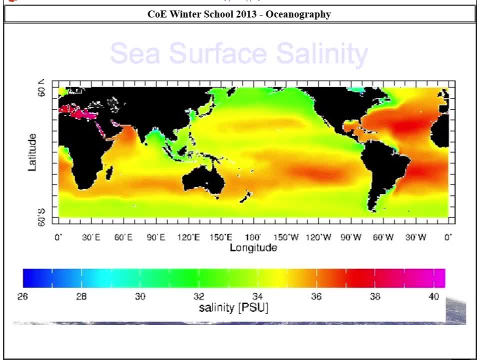 converging air masses in the mid latitudes. what makes air dry descent? exactly when you have air descending, it compresses. as it compresses, it warms. warm air can hold more moisture than cold air, so it's able to evaporate a lot. these are regions of net evaporation. 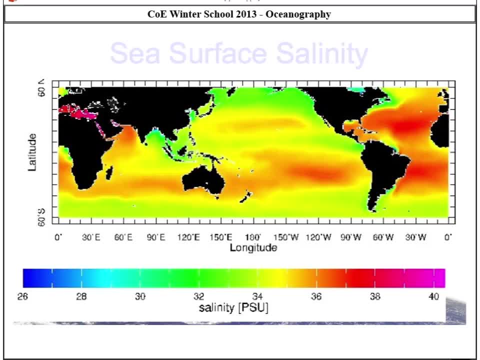 for sure. this is your descending branch in your happy cell. in the polar regions it tends to be a little bit colder. colder air holds less moisture than warm air and that's where you tend to have net amounts of precipitation. ok, next question: why is the Atlantic saltier than the Pacific? 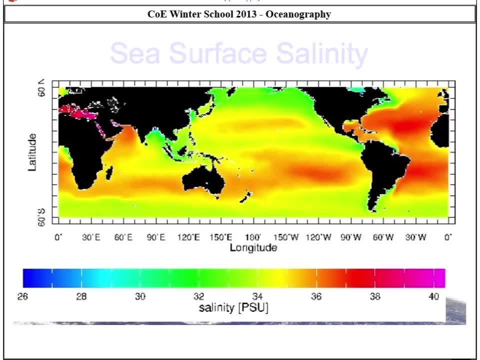 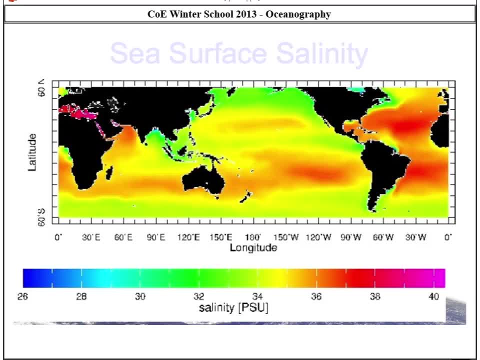 it doesn't have to drive very hard, does it to get over the isthmus of Panama? it doesn't have to drive very hard. there's a net moisture transport from the tropical Atlantic to the tropical Pacific across the isthmus of Panama. what about up here? 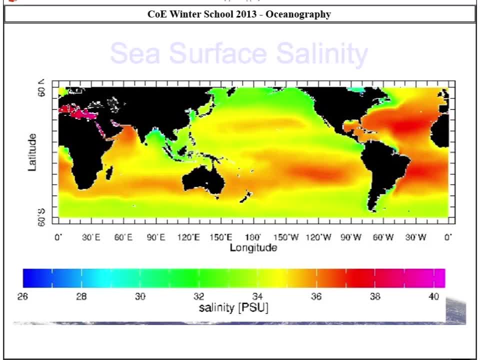 the winds are blowing this way right, it's hard to get over all of this land, isn't it? it's hard to get over all of this land, isn't it? so I think the simplest answer for why the Atlantic is saltier than the Pacific. I don't even know if this is hard or not. 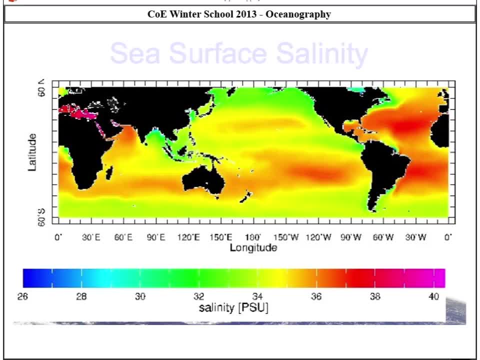 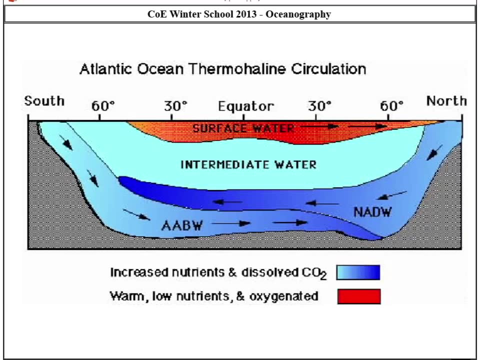 I just want to know for sure is that essentially, there is easier to transfer moisture across here than it is across here. ok, let's move on. ah yes, salinity with depth. one of the interesting things about the ocean is that, to first order, someone can go around with a bucket. 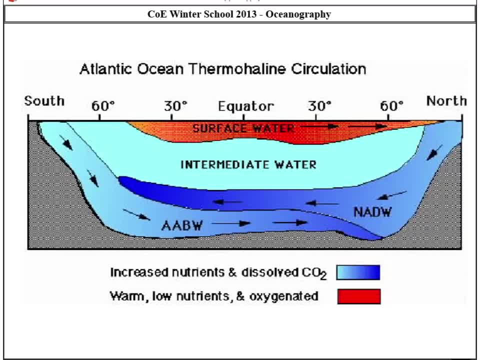 and put it deep into the ocean, pull the water out, measure its temperature and salinity and kind of tell where that water last came in contact with the surface. ok, So this is a schematic of the classical water masses in the ocean at depth Enter the bottom water last came in contact with the surface depth up there. 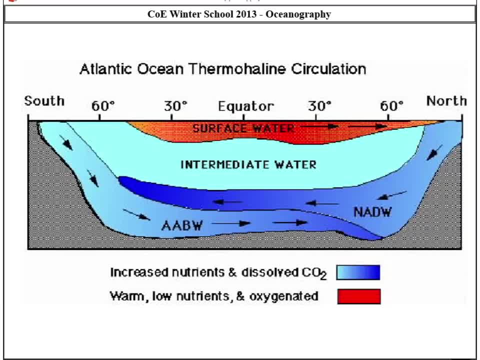 North Atlantic deep water formed up here, the warm surface water here. But essentially what this means? if you can identify this, trace this water, based on its temperature and sling, what does that mean for the interior flow? This temperature and sling isn't actually changing very much overall. 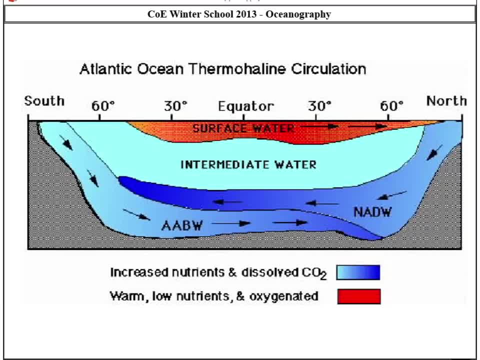 as it's flowing through the ocean, I think the word is it's largely adiabatic. It's essentially tending to flow along isotopicals, So these water masses are getting their characteristic properties at the surface flowing down at depth until they reach their 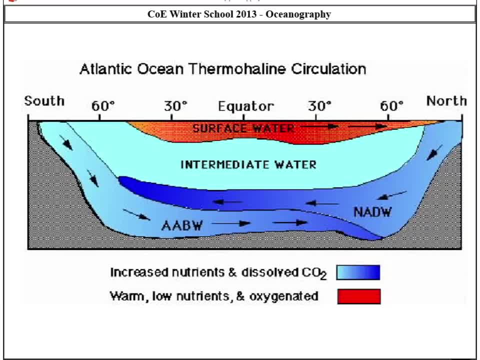 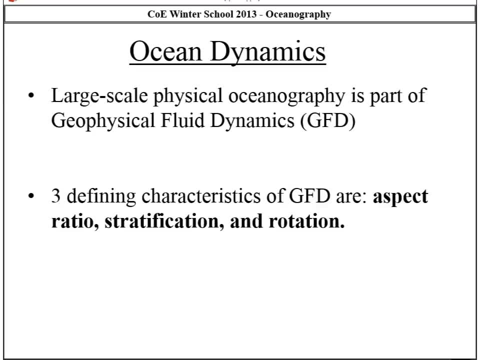 comfortable isopignal and then moving around the ocean along that isopignal. Now we're going to get into the more fun stuff- Geophysical fluid dynamics or the large scale physical oceanography characteristics- And we're going to keep it very nice and simple. 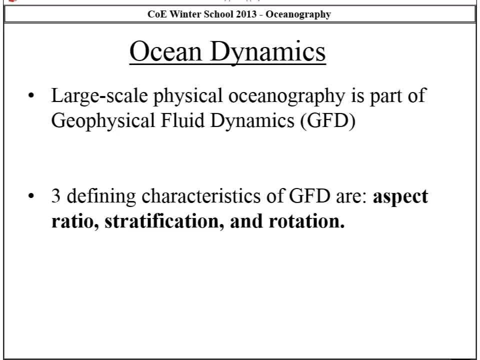 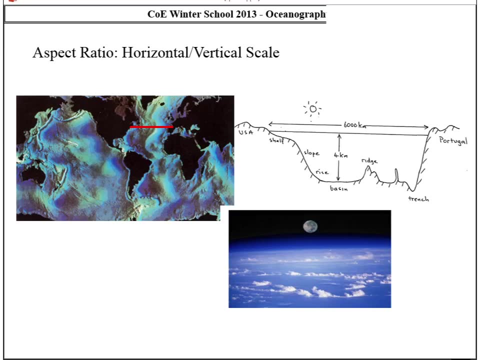 There are three, in my mind anyway, three defining characteristics of geophysical fluid dynamics. These are aspect ratio, stratification and rotation. What is aspect ratio? What is an aspect ratio? Anybody a photographer? I'm not. Yeah, weight versus the height, exactly. 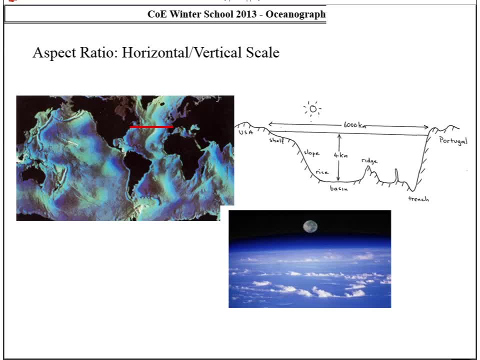 And so it's kind of the horizontal length scale versus the depth scale for the ocean. And so if you look at a place like the Atlantic or even on a larger extreme, the Pacific Basin, across the Atlantic it's about 6,000 kilometers. 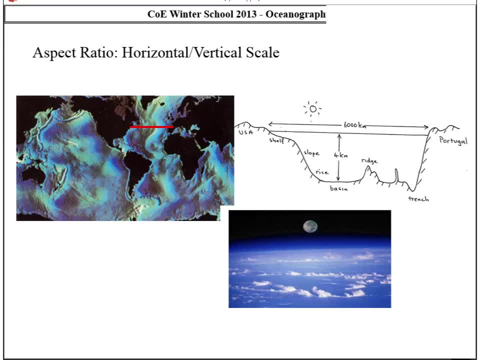 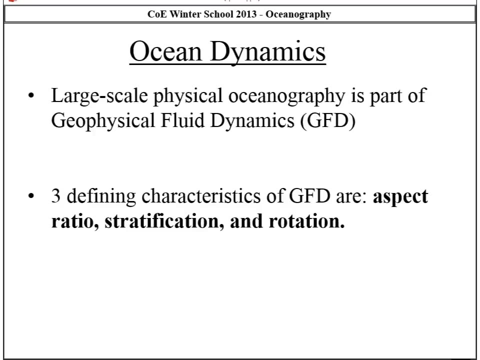 Your horizontal length scale, But your vertical length scale is like 4 kilometers, So its aspect ratio is huge. It's like 1,000.. And so when you see pictures of the ocean schematics like that, it's very important to realize. 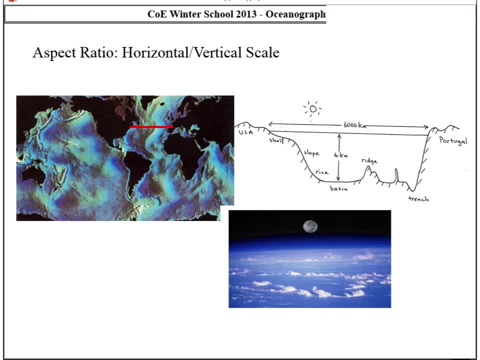 that that is a complete and utter lie. The aspect ratio of the ocean is pretty much the same as this piece of paper, Where this is your horizontal length scale and this is your depth. What does that imply about the ocean circulation? What sort of constraint is that going to put on oceanic motions? 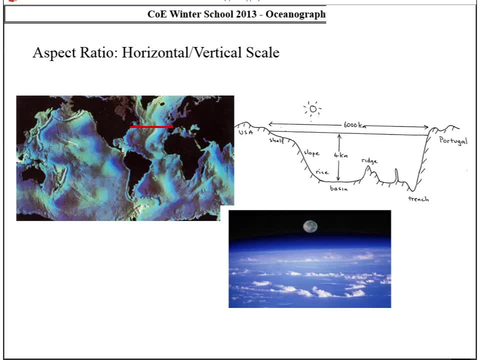 It's going to be dominated for the most part exactly by horizontal flow. This does not mean that vertical flows are not important. It just means they're going to be far less common First order Aspect ratio. It's true for the atmosphere as well. 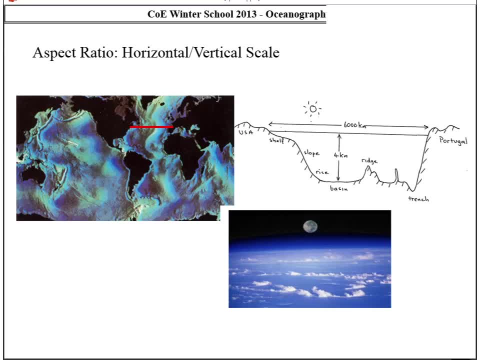 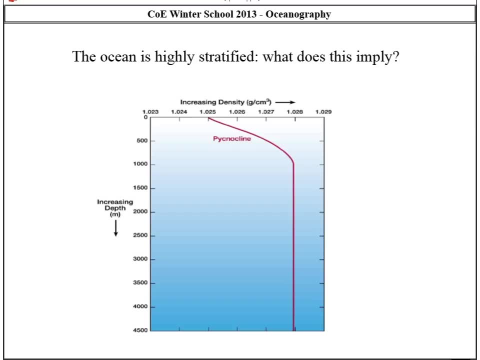 It's actually more true for the atmosphere, because it's all over the planet, It's not sideways. The next important thing for the ocean is stratified. This is a profile, a standard profile of density in the ocean: Less dense on the top, more dense as you go down. 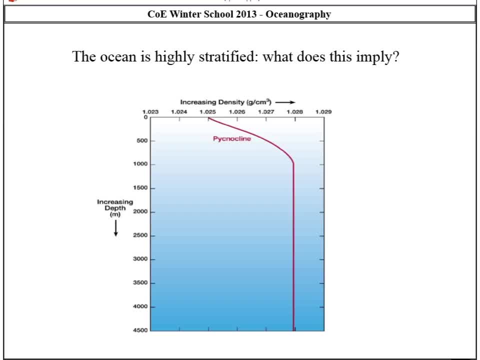 What does this imply? Stable, Stable, yeah. It's also going to probably kind of limit horizontal or vertical motions to a certain extent. Anything else, Where's the heat coming from The surface? The ocean is heated from the top. How is this different from the atmosphere? 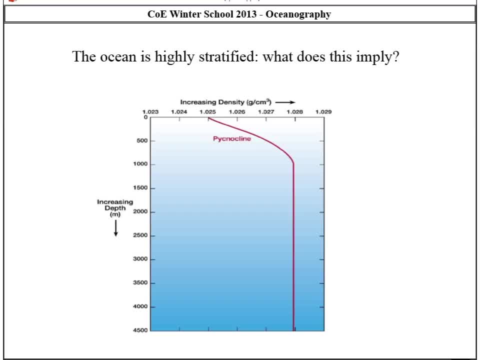 So where the curve becomes a straight line, basically is that where the client is. Yeah, this would be more called like a pycnocline, but it's the same idea. Yeah, yeah, Exactly, yeah, Okay. so it's warmer at the top and maybe fresher a little bit. 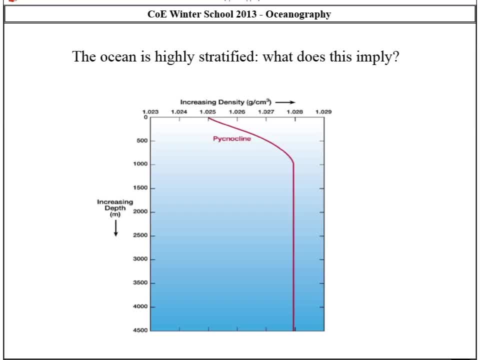 So it's essentially telling us that the ocean is heated from the top. How is this very different from the atmosphere? Where is the atmosphere heated from? for the most part, From the bottom, From the bottom. What are you going to have a lot more of in the atmosphere than in the ocean. 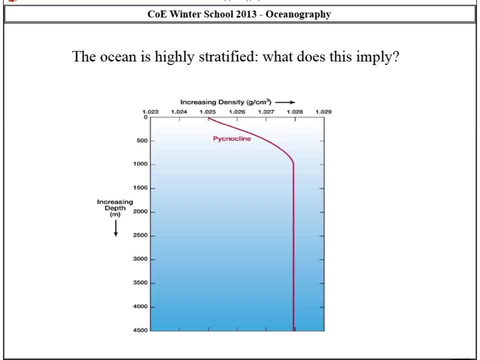 Convection, Convection- yeah, You're going to have a lot more active convection in the atmosphere than you have in the ocean. You still have convection in the ocean and it is very, very important, but it tends to be highly localized. 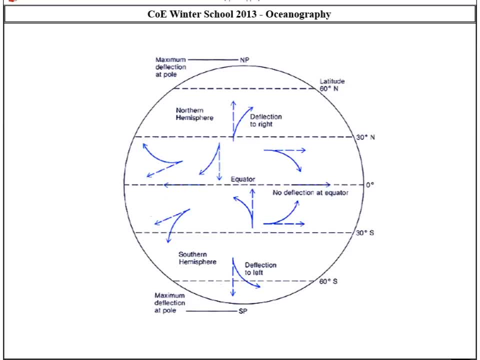 Next one, my favorite, is the rotation. What is this thing called? What is going on here? The Coriolis force, Everybody's favorite. Is it true Or is it fake? It's fictitious. What does fictitious mean? 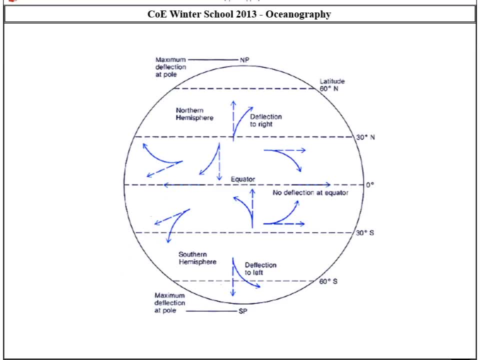 It goes back to Newton. It's all Newton's fault. You can spend. I used to do a two-hour lecture on the Coriolis force and I actually think it's still kind of an active part of research. I'm going to do it now, in two minutes. 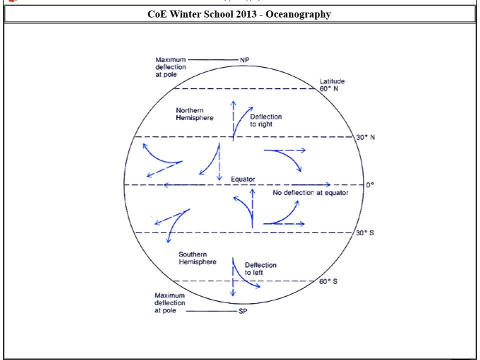 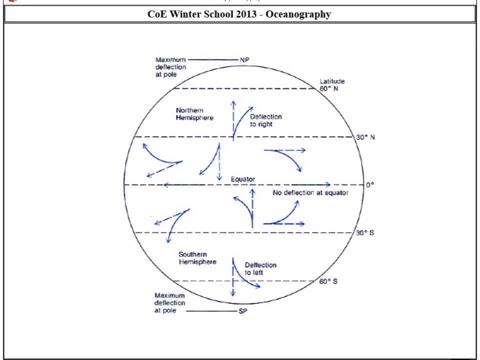 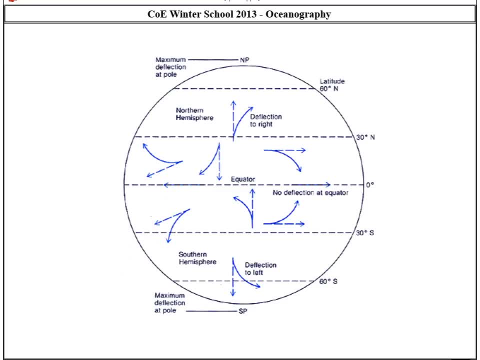 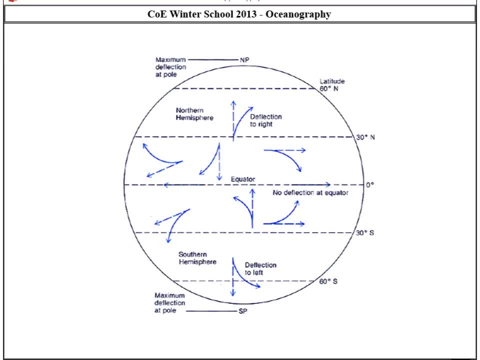 In the northern hemisphere. a turntable world is rotating that way: Flat Earth. I am now an observer fixed in outer space, observing planet Earth, watching a parcel here. Yeah, This parcel is rotating, It's fixed, It's not, you know, moving relative to this spindle. 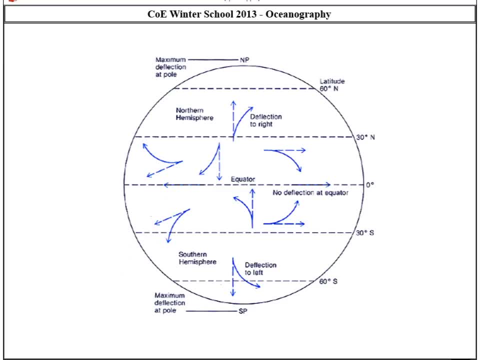 but it's still rotating around, just like on a record on a turntable. Is this parcel accelerating? Yes, Why is it accelerating? It's changing its direction. It's not changing its speed, its angular speed, but it's changing its direction. 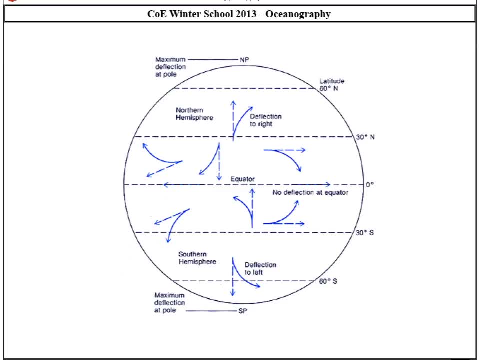 This parcel is accelerating. Newton tells us that there must be force acting on it. What is the force acting on it? Let's imagine that this is a parcel. So this is my parcel, And it's rotating, It's changing its direction. 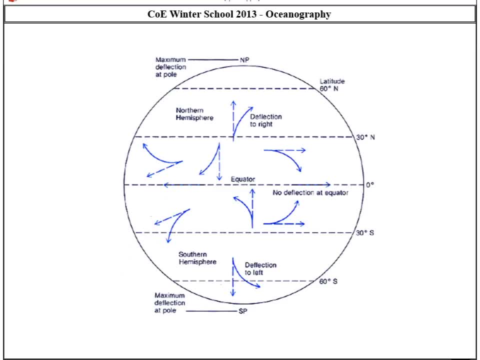 It's accelerating. There is a force. The force is the tension on this, and you know the rope, the string. What on planet Earth? It's your centripetal force, this one. What's the centripetal force or acceleration on planet Earth? 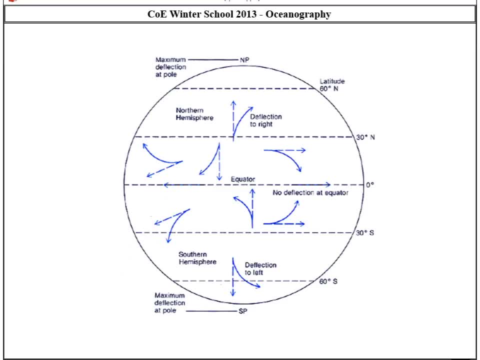 Why are you not flying off in outer space? Gravity, Gravity. So, from the viewer in outer space, there is a force applied to maintain the acceleration. That is the force of gravity. Acceleration is not equal to zero and there is a force of gravity. 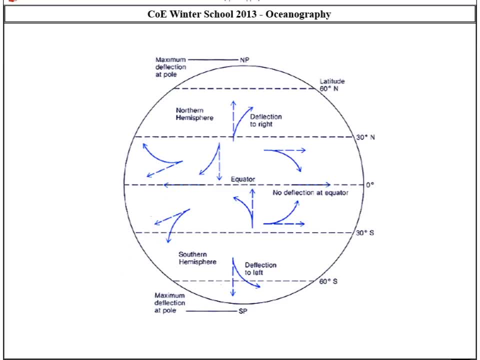 Check. Newton was correct. Now let us put the observer on the Earth. They're all both rotating. Yeah, Does this person see this thing accelerating? Nope, Not accelerating. Now, the acceleration is equal to zero. Does that mean there is no force of gravity? 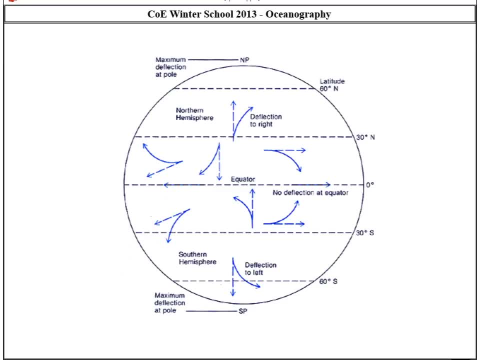 The sum of all forces must be zero if there is no acceleration. But we still know there must be a force of gravity. Right Hence we came up with the centrifugal force, So that when we applied Newton's laws to a rotating frame of reference, 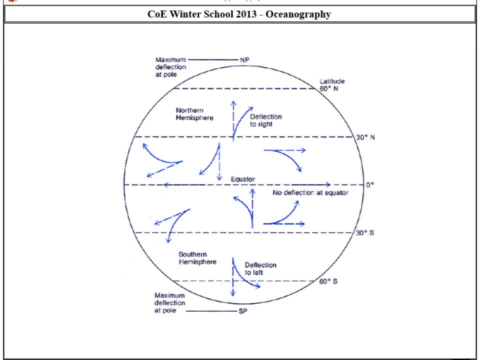 a non-inertial frame of reference, they still work. OK. Now if this parcel here starts moving faster, starts moving relative to the turn table, then you need to have the Coriolis force to maintain Newton's laws. Let's watch a movie. 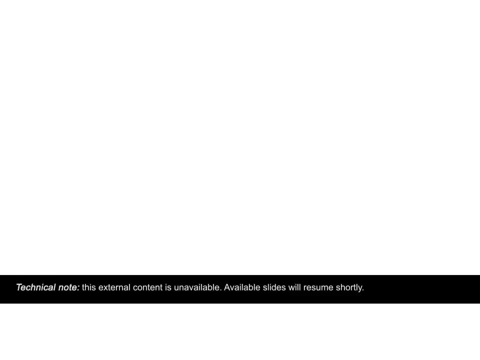 Movie is here Here. I like this one. It's really short so you can be quick. How do I do it? Full screen. To an observer above the merry-go-round, the path of the ball appears straight, while to someone sitting on it. 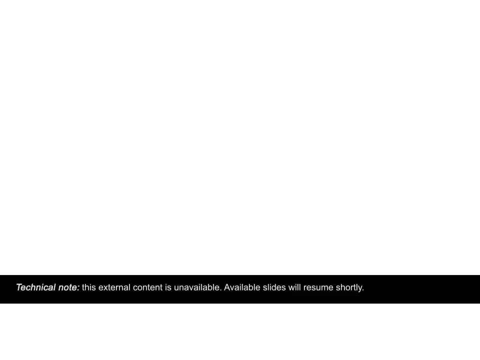 the ball appears to curve to the left. This exemplifies the Coriolis force whereby, to an observer on the rotating Earth, the path of an object appears to be deflected, and this is a result of the Earth's rotation Happy. 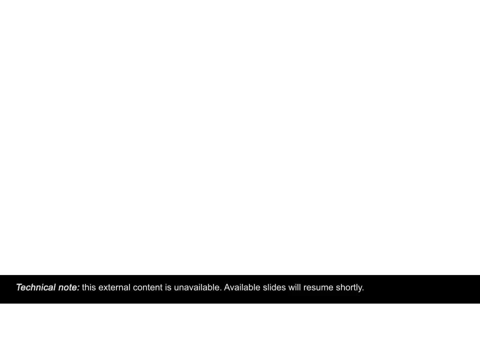 Are there other questions? There's other ones. I really like Other videos. All right, we've got to move forward. OK, Slideshow, Slideshow. Is that a tool? OK, I'm going too slow, We're going to speed up. 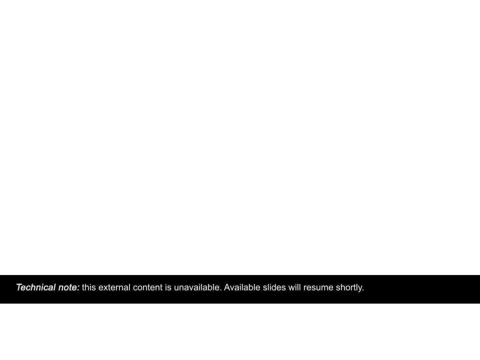 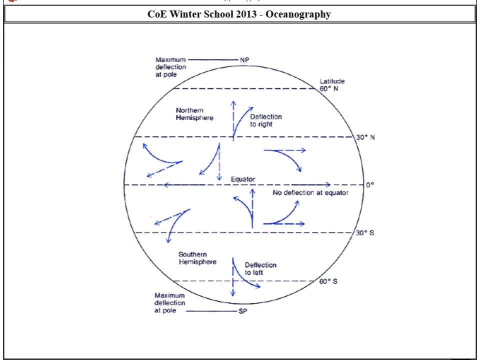 It's fun. It's fun, It's fun, Oh yeah. Does the Coriolis force apply everywhere? How do we know when it's important? When do we know it's important? Catch Ooh, It bends, Sorry. 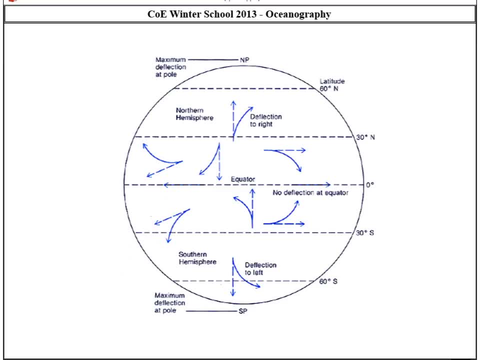 I should have warned you. Sorry, Sorry, Sorry, Sorry, Sorry, Sorry, Sorry. Does it bend, Ready, Ready? Ah, It's pretty straight. It's pretty straight. Why didn't it bend? When does it matter? 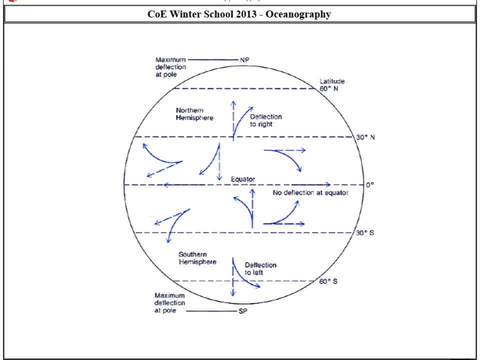 When does it matter? That's because of the distances and the speed. It's a question of how – so the rotation timescale is 24 hours, right? T is equal to 24 hours, So you can kind of think of it. if a particle gets estimated to be, 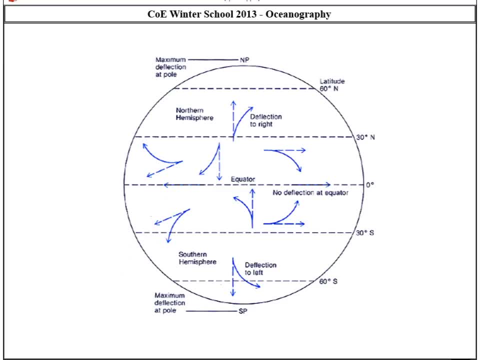 say 24, or if a particle is supposed to be that wide, a current, an atom or something like that, what is going to happen if a parcel is moving at a certain velocity, over a certain distance, with a certain over a certain velocity? that gives you time. scale time right, if that. 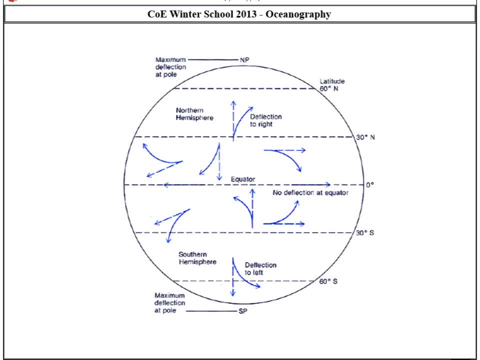 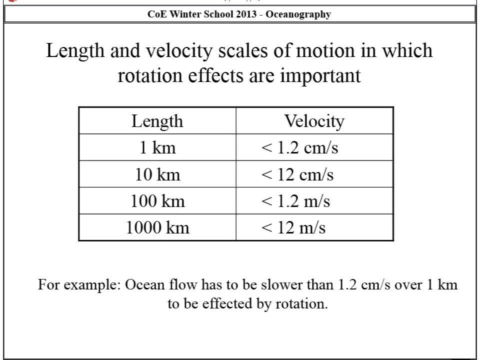 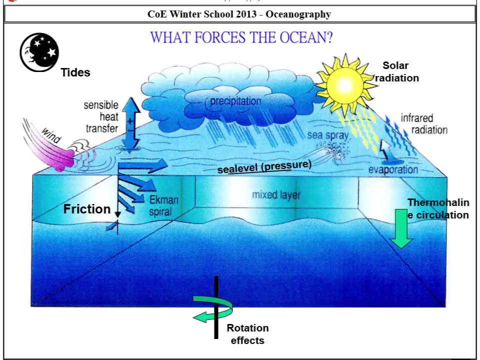 time is roughly equal to 24 hours. that is important, so for the atmosphere and the ocean, so for an ocean. flow is typically moving at speeds like this, so we're. distances like this does not matter for toilet bowls. well, I found an awesome video of someone taking toilet bowl. photos of Australia and Canada, okay. 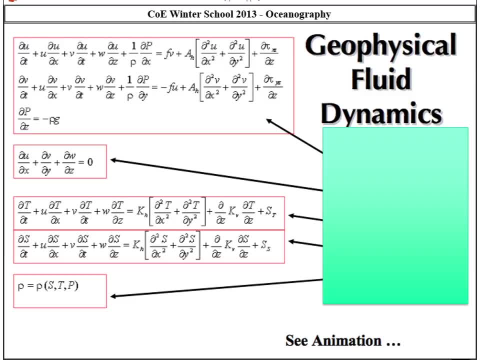 we're gonna move to this one, everybody's favorite- geophysical fluid dynamics. if you want to be, you know, master of the universe, you need to solve seven equations for seven unknown variables. these are your seven equations. seven unknown variables are UV and W, your velocities, temperature, salinity, pressure. 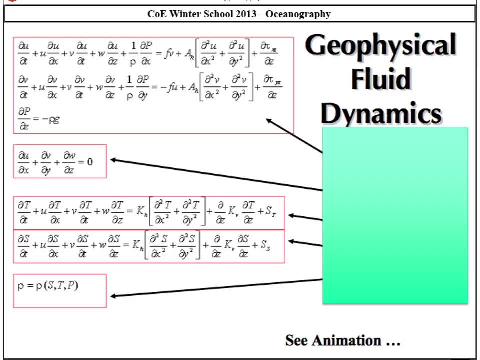 and density. okay, these are all based on physical laws. what are the physical laws we're applying here? conservation of mass, conservation of momentum, other ones, yeah, that's sort of the conservation of mass. yeah, exactly, conservation energy, that's the conservation momentum. your conservation momentum is: gives the three of them UVW. 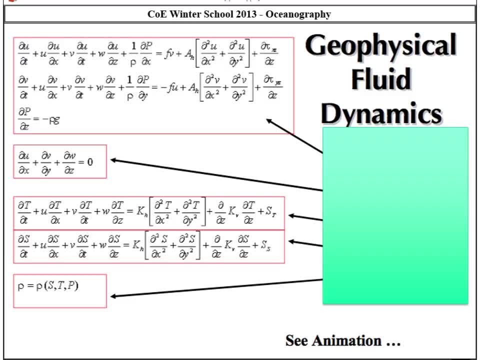 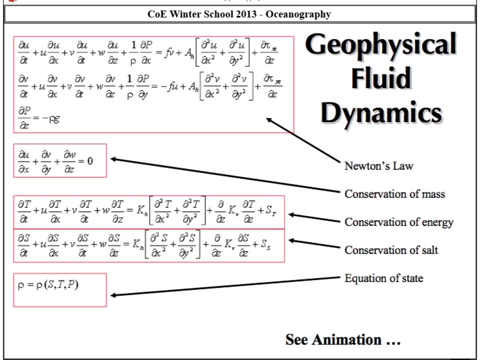 this for conservation of energy: gives five concentration of salt and stay baby. oh, you just think that's right. that's right, love them. yeah, what's going on here? you, F equals ma. conservation of momentum, F equals ma. this whole point, stuff. here is your a term, that's your acceleration turn fluid dynamics. okay, we'll go. 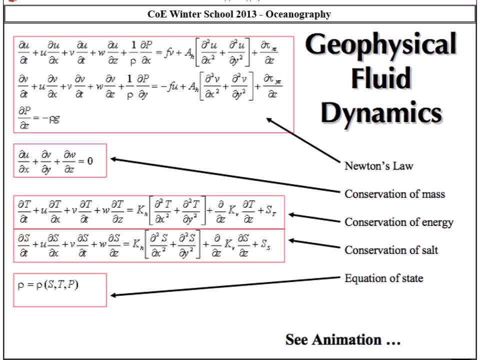 through that a little bit. I know you love it. this here is one your primary forces. so a is your acceleration. everything else here, your forces, that people that make this is your pressure. gradient pressure as a force, dp by dx. This is your Coriolis force. 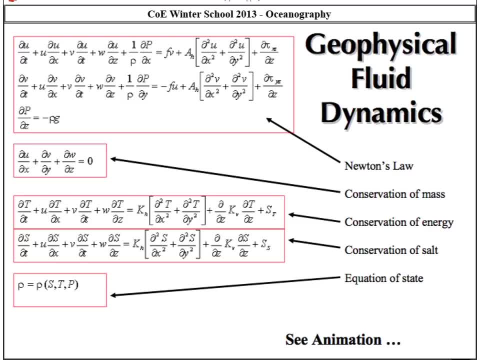 Notice that the Coriolis force is dependent of the v, the north-south velocity for the u equation. How interesting. Then you have friction and this is the winds over there. That's sort of what we're going to break down. 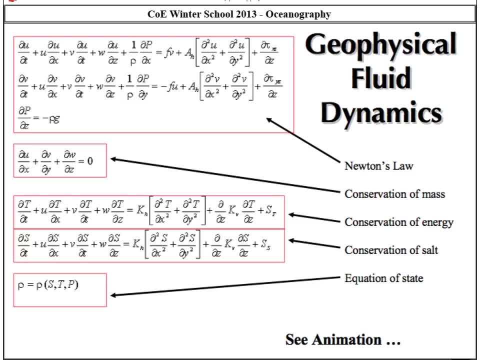 East-west momentum equation. north-south momentum equation: same idea, but notice the v is dependent on the u Coriolis force. This is your, w your vertical velocity equation. Notice there's no w in it. Why is there no w in it? 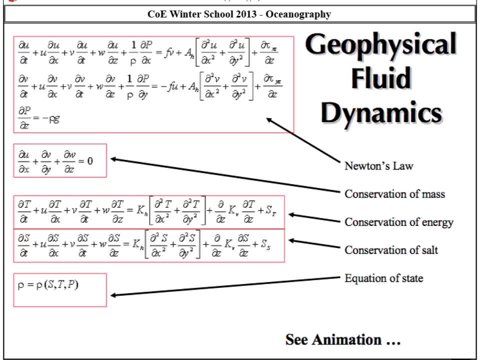 Sorry. so obviously people use quadratic viscosity and stuff, blah, blah, blah, and they use it for numerical modeling reasons. Obviously, at molecular scales you have friction and people use- They use four-portal viscosity and they use all sorts of different things. 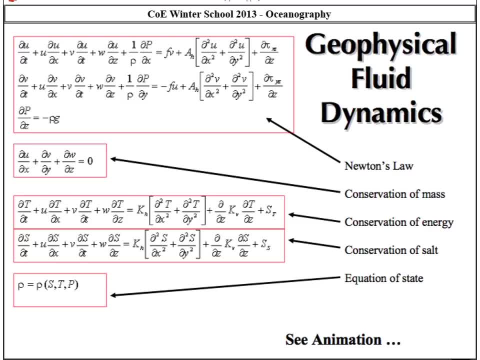 Is there any reason to assume that viscosity is quadratic or anything else? No, It's just dependent on what kind of questions you want to answer, what kind of questions you want to address. There's no doubt: the devil is in the details. The devil is in there, for sure. 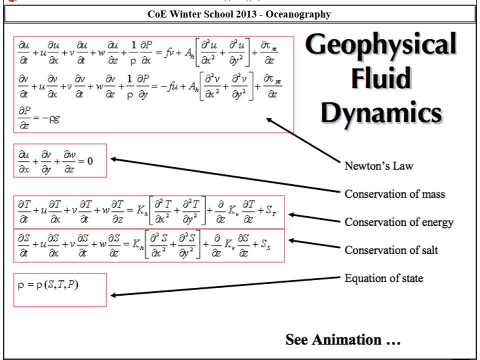 Ties. this is not really shown in here. That's all being hidden in there. It's totally true. It really depends on what kind of question you want to address. It's really the modeling, you know, global climate modeling version of this equation. 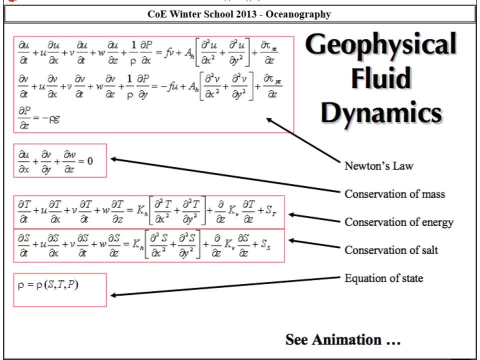 Yeah, no, it's a great point. Where's w For this equation? here we're kind of ignoring it to a certain extent. Okay, we're saying that for the large scale. overall, except in special places, there's not a lot of w going on. 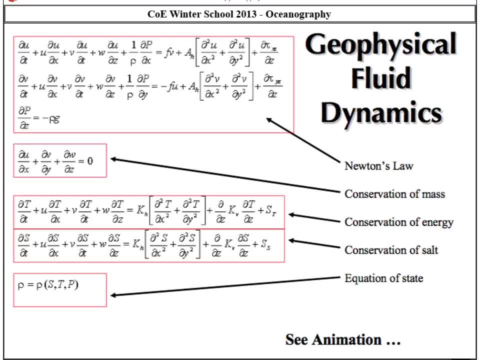 This is your funny little conservation of mass. Okay, but it's really for the ocean. we sometimes deduce it down to saying it's conservation of volume, And what this equation is really saying is, if you take a blob of water, the amount of water moving into that volume has to equal the amount of water going out of that volume. 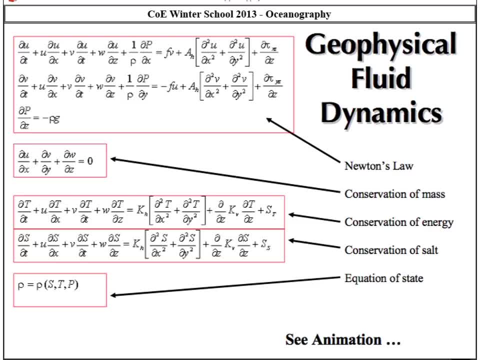 Okay, And then this is your thermodynamic conservation of energy. Again, this is sort of your a, you know your advection or your acceleration of heat. Okay, your advection of heat, And then on the other side it's just sources, sinks and friction, but here it's called diffusion. 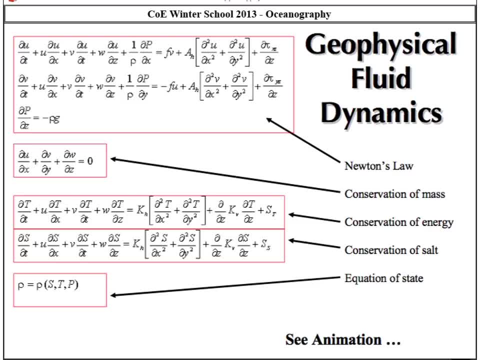 Okay, so how heat is diffused horizontally and vertically, And then your source terms. So whatever, solar heating, latent heating, all that other stuff. Okay, Same idea for salt. It's pretty simple: Advection of salt, diffusion of salt, and then sources and sinks. 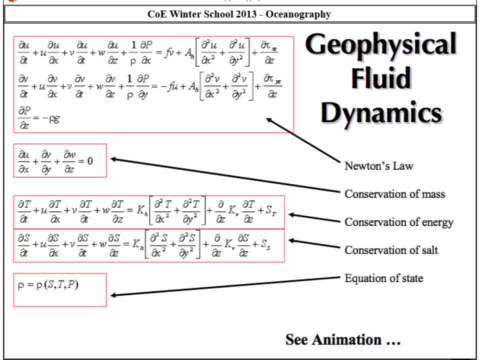 Again the devils in the details, right The sources and sinks and the diffusion processes Totally, And then the equation of states, So relating density to salinity, temperature and pressure. Sounds easy, but then Trevor McDougal comes along. 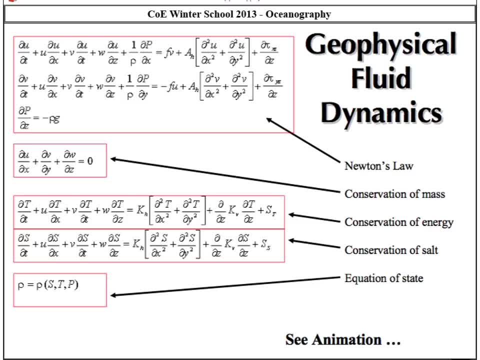 Okay, This is still in computer models. this is the one that takes up the most amount of time. It's a total pain. And then you know we still don't. Trevor McDougal, It's a little pain. 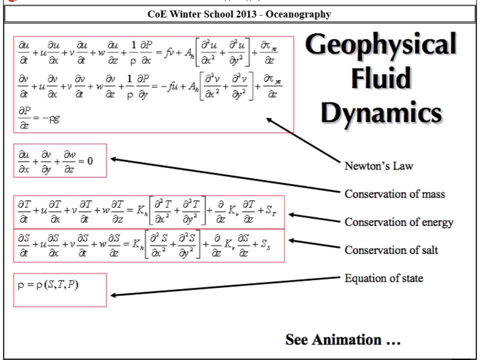 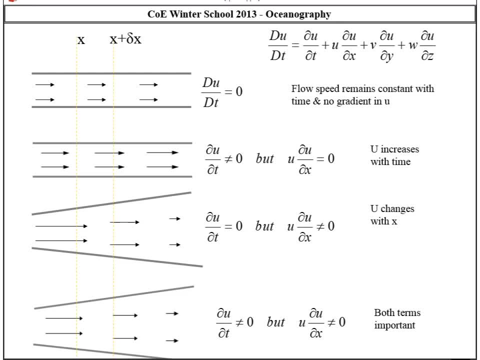 Uh Yeah, let's look. Okay, we gotta keep moving. We're gonna deal a little bit with this acceleration term. I'm gonna put a hole there. Acceleration term: The material derivative. Awesome, The Lagrangian derivative. 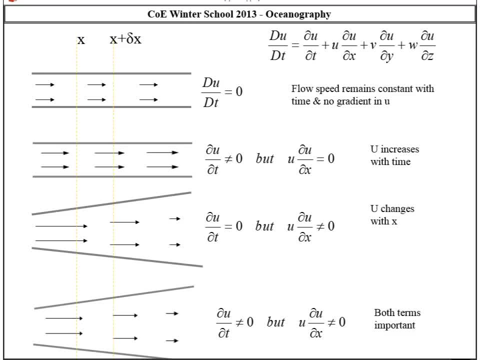 Whatever All this stuff right. d by dt plus u, d by x plus u, blah, blah, blah. Let's just deal with the? u terms here. okay, I think this is awesome. Alex and Gupta gave me this slide. 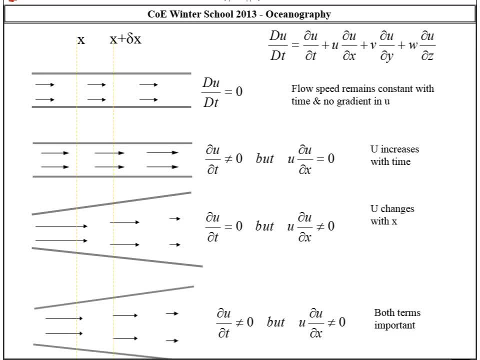 Okay, This is your x direction Across here. Notice, in this example, nothing's moving. Nothing's changing in the x direction or with time, Which means that du by dt, the big du by dt, the whole shebang is zero. 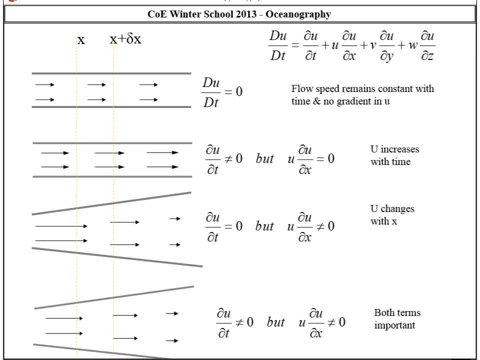 Okay, Easy Now in this one, at any individual time, the velocities are the same, no matter where you are in the x direction. Does that make sense? So the du by dx term is zero, But the velocity at a specific point is changing in time. 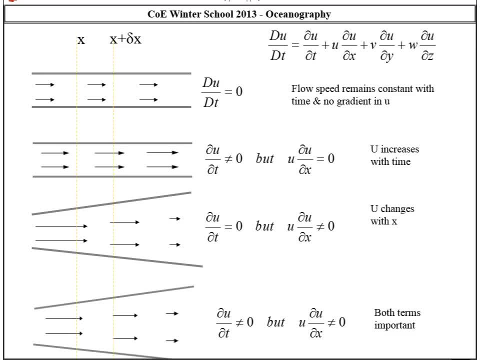 Okay, So the du by dt term here is not zero. It is an acceleration, And I think of this. I used to kayak rivers a lot in the past life And I think of this. as you know, you're going down a river that's moving on its own at a constant speed. 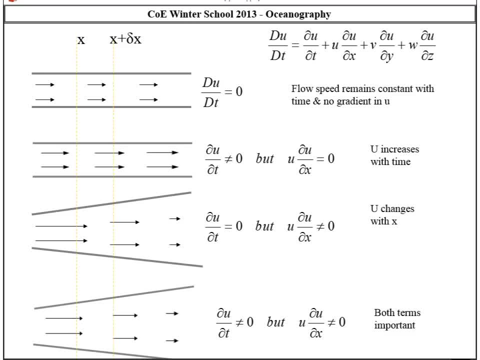 But then I start paddling relative to the river, No problem, That's what's happening here. You could also imagine a river where I'm just being lazy and floating down- I'm not paddling, But it's changing its width. And as the river changes its width, its flow changes speed. 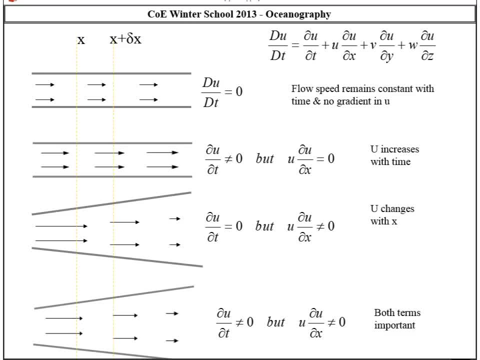 So in this case there is no change with respect to time, But there is a change in the velocity with respect to your position. Okay, The lazy paddler just going down a meandering river. So du by dx now is not equal to zero. 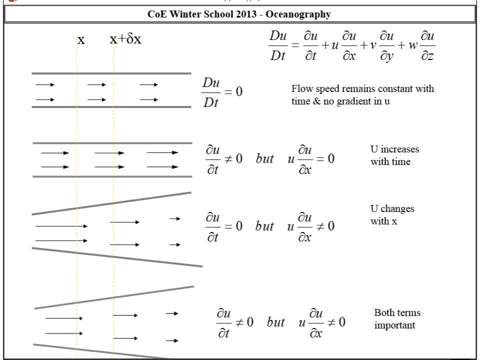 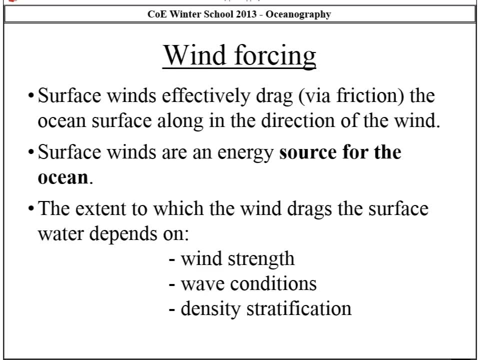 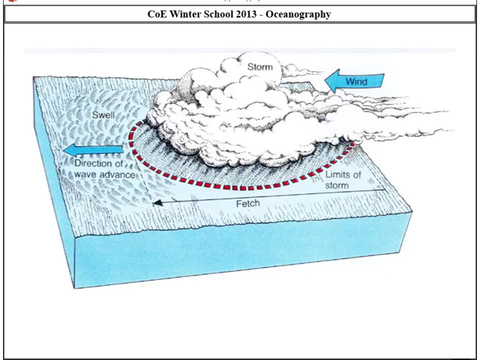 That's those other bits. Happy, Good. Okay, Wind, you know this kind of gets boring, but wind blows on the ocean. Wind is supplying energy. It's a source of momentum to the ocean. Yeah, That's good. 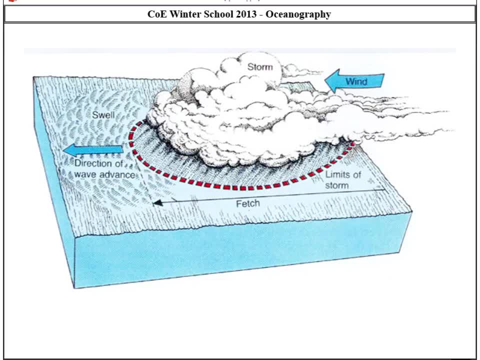 That's right at the surface. As you go down deeper into the ocean, the main stress kind of just behaves like friction. Okay, The amount of impact that the wind has on the ocean is dependent on a few things. It depends on how strong the wind is blowing. 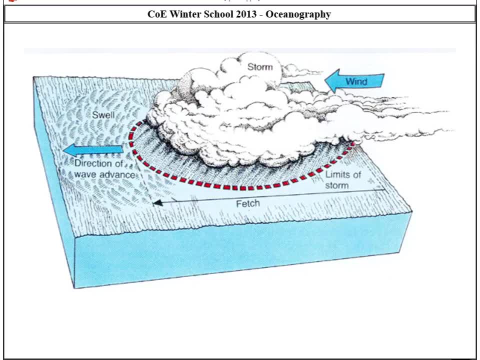 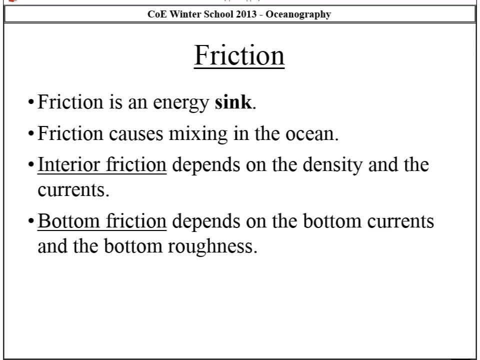 It depends on the length over which that wind is blowing, Okay, Oh, and on the stratification of the ocean as well. So how stratified the layers are, Friction is really an energy sink in the ocean. Okay, It's dissipating energy. 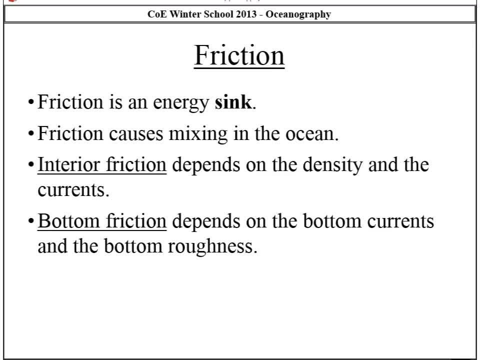 It always wins. You can imagine two types of friction: An interior friction, so you know, away from any boundaries, away from the top of the ocean, and away from the bottom of the ocean, The interior of the ocean, I think for the most part. 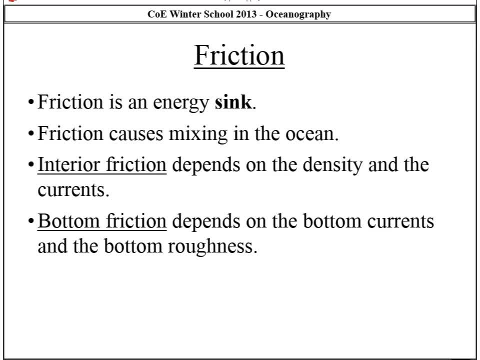 you can consider to be inviscid. It's quite very, very weak. Okay, Interior, there's not a lot of interior friction in the ocean, It's largely inviscid. Bottom friction is more important. So when you have a flow over rough to thin tree, 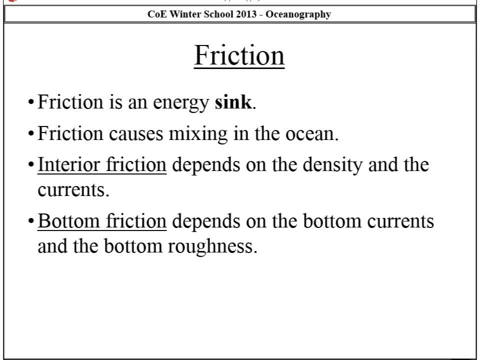 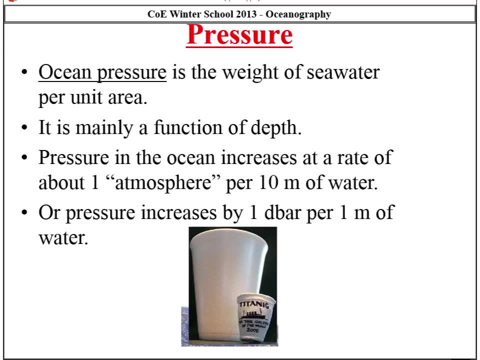 Like tidal currents or really really strong deep currents. Those are going to have friction with the side, with the bottom, Just like you have wind friction at the top. Okay, The next one we want to talk about is pressure. Pressure is just the weight of the column of fluid above you. 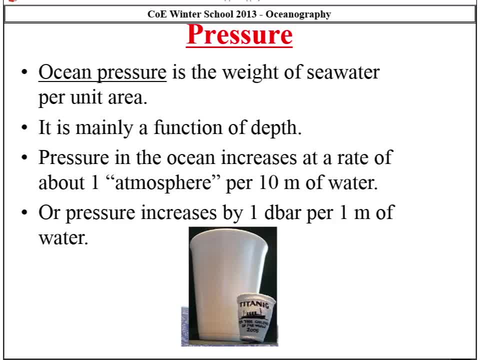 P is equal to rho gh. So right now I we're all feeling pressure From the weight of the atmospheric column above us. As you go deeper into the ocean, Water's heavy. You feel more and more pressure. So about 10 meters down you've doubled the atmosphere. 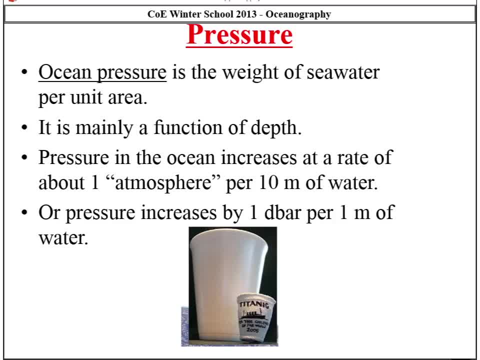 It's twice. You've added like another whole atmosphere on top of you. The interesting thing about pressure is that it acts in all directions. So if you take a styrofoam cup down to the Titanic, it maintains its shape Okay. 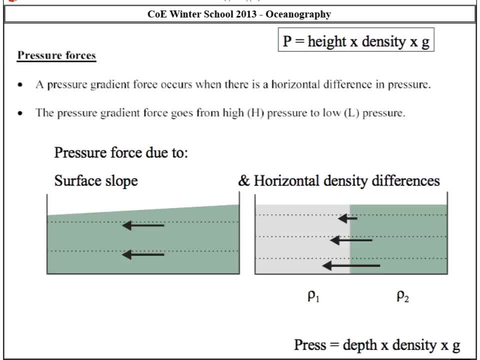 Yeah, Yeah, Okay, A couple different types of pressure forces. You can imagine one scenario where the whole ocean in this thing is one density. Okay, It has this fixed density, But there's differences in sea surface height. Okay, So there's more water here than here. 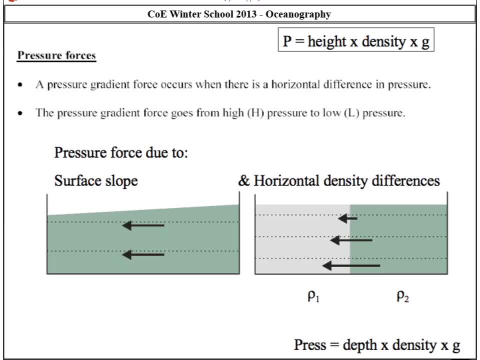 And so if you're down at this point in the ocean, this dude is feeling the weight of the column of fluid above him And this dude is feeling the pressure of the column of fluid above them. here, This dude's feeling more pressure. Yeah, 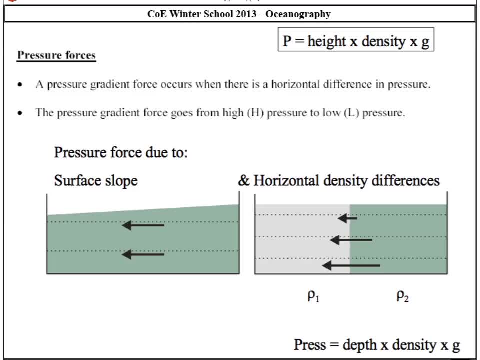 Hence the pressure gradient. The interesting thing about this scenario is that, as you go down into the column, the pressure gradient force is constant, It doesn't change with depth, And that pressure gradient force is only due to the difference in sea surface height. 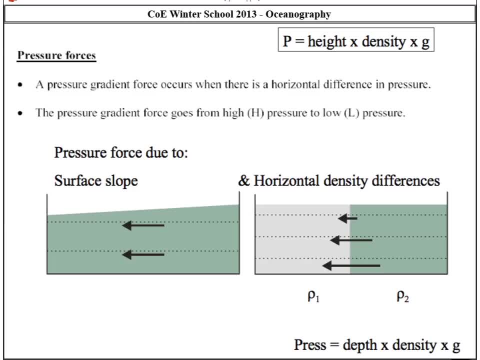 This little bit of anomaly here. Okay, It doesn't change as you go down. You can imagine another scenario here where the ocean surface, sea surface height is fixed, It's flat, But one side is more dense than the other. And in this scenario, 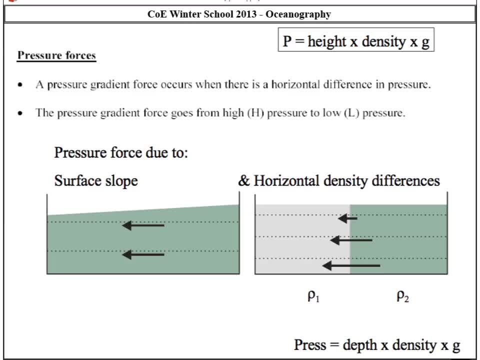 the pressure force increases with depth Because there's a cumulative effect of this rho g, h pressure used with depth times, density times g. This density difference continues to accumulate as you go down. Does that make sense? What is the fancy words for these two types of flows? 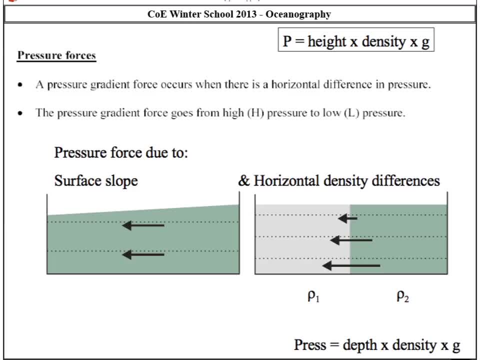 Pressure driven flows. Hmm, Hmm, It's barotropic and baroclinic. Yeah, This would be barotropic flow and this would be a baroclinic flow. This is not always this simple, But it's a good way to break it down. 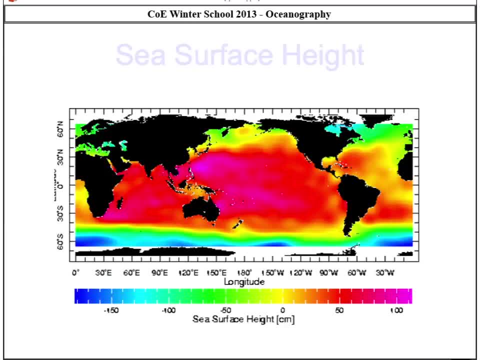 Okay, So with the satellite this is a sea surface height over planet Earth. So we have high sea surface height here and low sea surface height. People can go around with satellites now and look at changes in sea surface height And then from that. 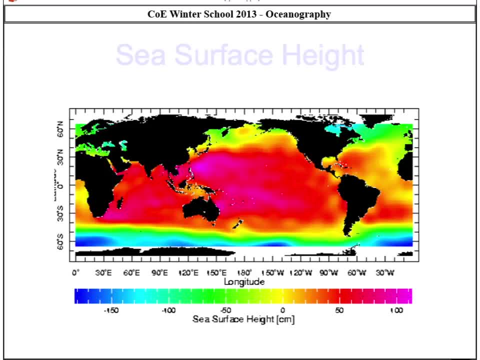 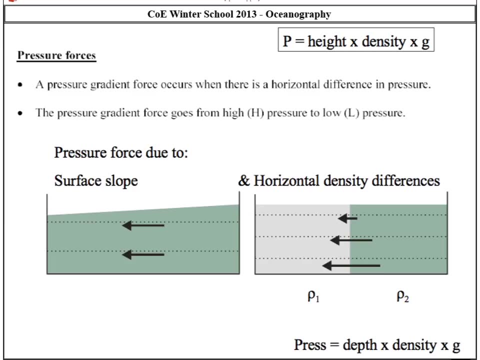 deduce a pressure gradient. Okay, Well, what type of pressure gradient does this tell you? Hmm, Is that giving you this one or this one? It's giving you the first one? Yeah, It's giving you the barotropic component. 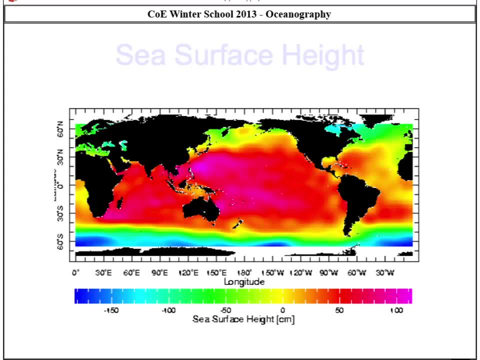 It's not totally that simple, but we've got an hour Back in the old days, before we had satellites, they'd just go around with their satellites, They'd go through the bucket and measure this stuff And then they'd assume that the sea surface height is flat. 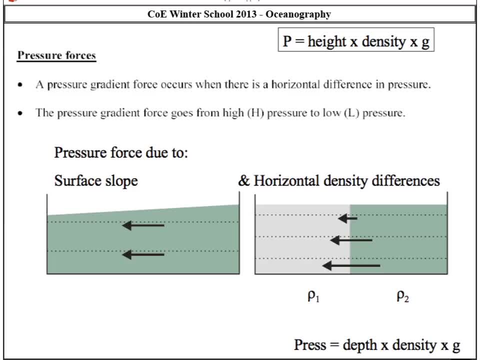 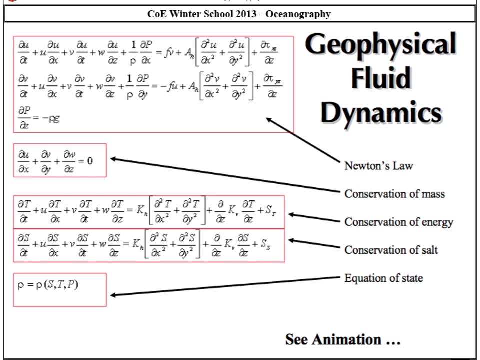 And they'd only get the baroclinic part And a good old fix. Okay, Right, So we're going to talk mostly about finish off, really just looking at these two, just the horizontal momentum equations, Okay, And look at some of the basic stuff. 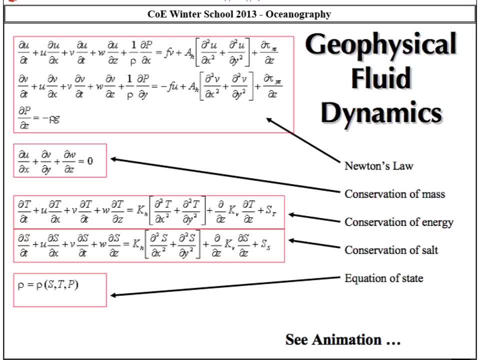 that come out of these horizontal momentum equations. It's a complicated equation, But you can really say that only certain parts of that equation are important for certain parts of the ocean. Okay, And so we're going to start with wind forcing and rotation. 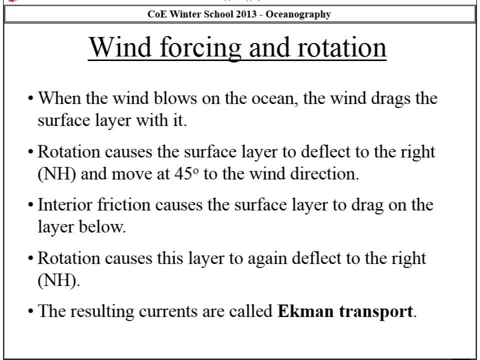 So when you're at the surface of the ocean or in the upper couple hundred meters, the only two parts of that horizontal momentum equation that really matter are the wind forcing, the wind stress and the Coriolis force. Those are the dominant terms at equilibrium. 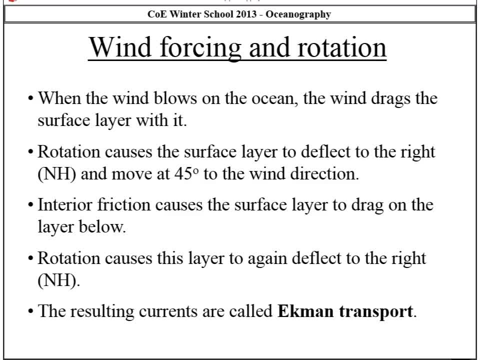 At equilibrium, meaning there's no acceleration. Okay, We're at steady state. So wind forcing and rotation. Okay, Let's imagine the wind is blowing this way in the Northern Hemisphere. Okay, I'm a parcel of water, I start moving with the wind. 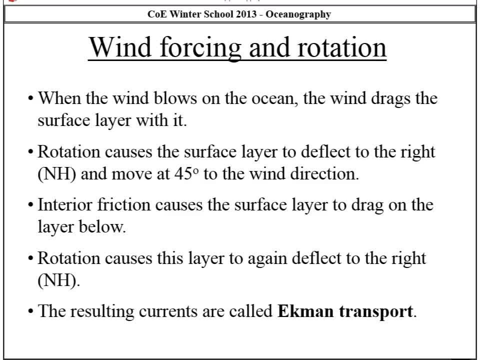 in this direction, in the Northern Hemisphere- I'm saying Northern Hemisphere because I can, only it's not very much of a movement. If I start moving in this direction and that rotation kicks in, what's going to happen to me? I'm going to get deflected to the right. 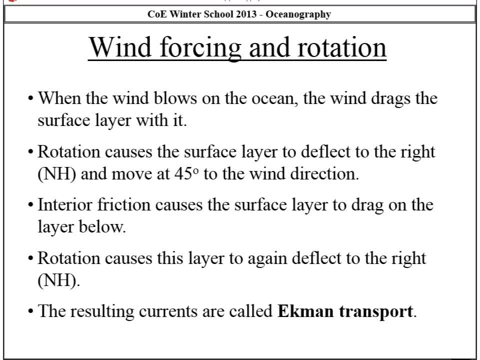 Start moving, get deflected to the right, Exactly Okay. Now let's imagine that was the particle on the top. Let's imagine now that I'm a particle one layer below. I'm that particle one layer below And I'm feeling. 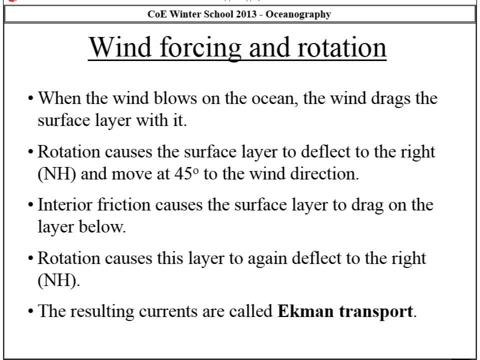 essentially stress from the layer above me. Yeah, So now I'm moving in this direction Like the wind's blowing. it was really just friction. I'm moving and what's going to happen? I'm going to get. I'm going to get. 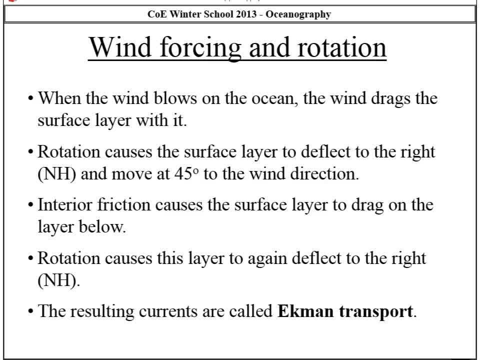 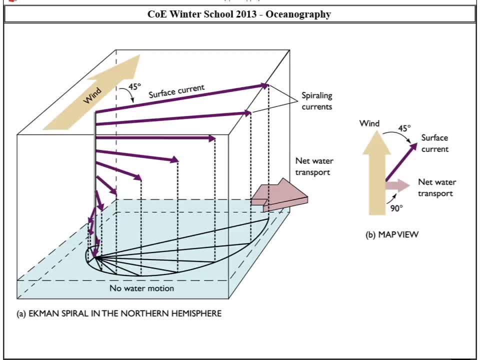 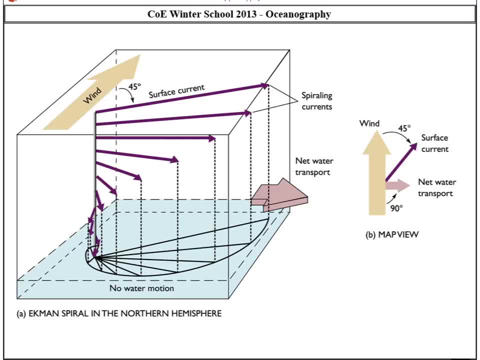 Okay, So the wind blows in this direction. in the northern hemisphere, the core will, of course, deflect to the right. As you go down the layers. it keeps happening, just friction, layer by layer and layer, until all the energy's dissipated out. 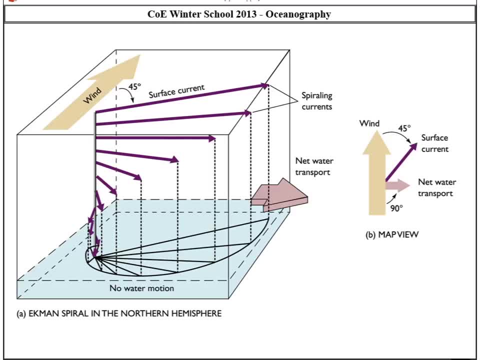 Okay, If you indicate over this whole wind-affected layer which is depending on how strong the wind is and all that other stuff, you know it's at 50, a couple hundred meters If you integrate the net transport over that whole column. 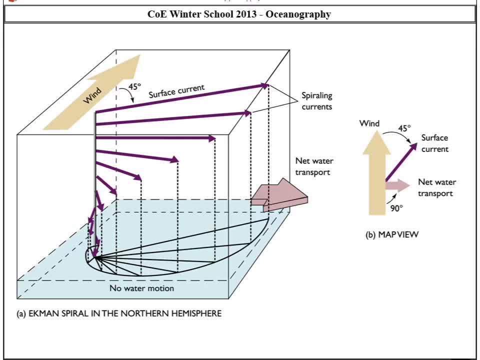 the net transport is 90 degrees to the right of the wind. Okay, So if the wind's blowing this way, your net Ekman layer transport is to this direction, Which brings me to one of my favourite stories in oceanography: Uh. 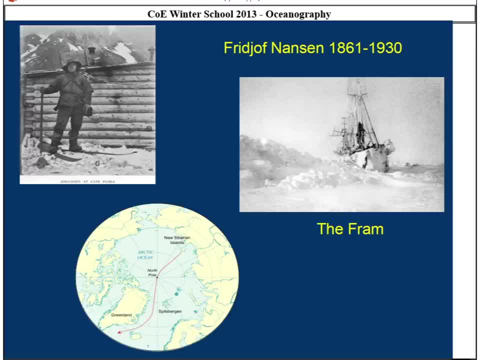 Friedhof Nansen. Who's heard of Friedhof Nansen? Yeah, he's such a dude For so many years, for so many reasons. Yeah, when he finished grad school, his PhD, he was like the first guy to walk across Greenland. 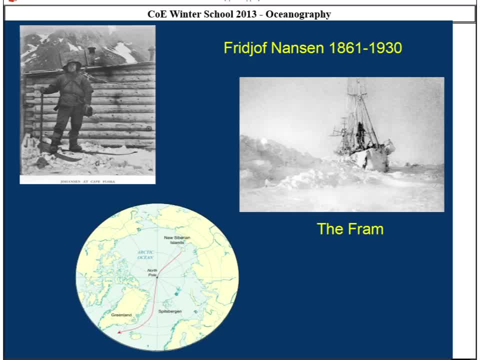 which you might know is covered by, you know, three kilometres thick of ice. He then decided in his late 20s that he wanted to be the first man. he's Norwegian, he died in 1930, he wanted to be the first man. 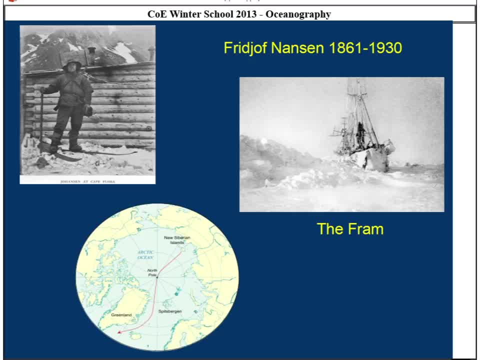 to get to the North Pole. To do this, he convinced a bunch of people to build him a boat called the Fram, Which I believe means forward in Norwegian. Uh, the idea was to build this really weird boat and it actually had tree trunks. 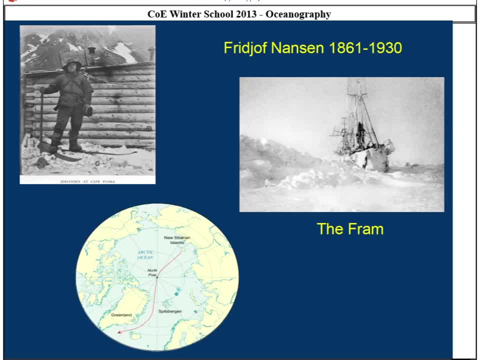 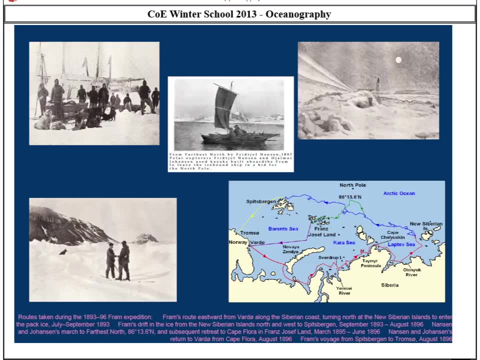 as a like. it's core was made with really strong tree trunks To drive this boat. I'm going to give the very abbreviated version: Get the boat doesn't sail very well. sail it over here. They had the idea that if they locked it. 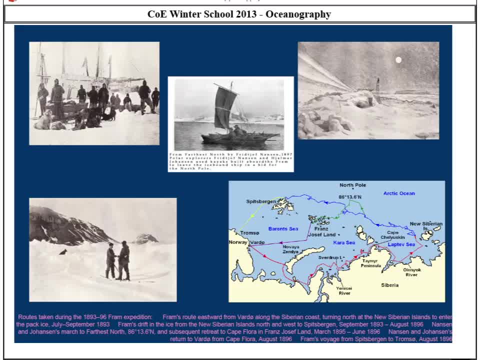 into the ice here. the wind would just sort of blow them over the North Pole. So they got 12 guys and 5 men and they built a boat that was actually 12 guys and 5 years food. I know It's so insane. 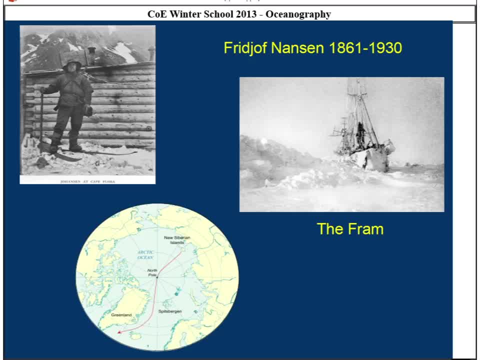 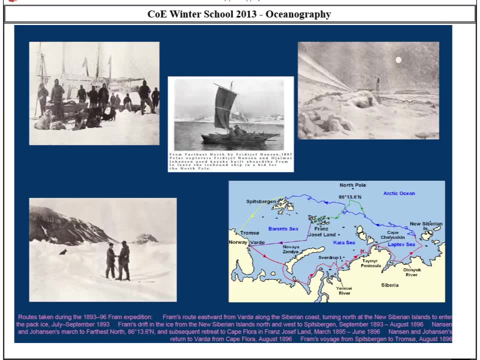 One way to get somewhere insane: Ram the boat into the water, Into the sea ice, And hope for the best. Uh then they did like this big pattern for like 6 months and came back and were like we're behind from where they started. 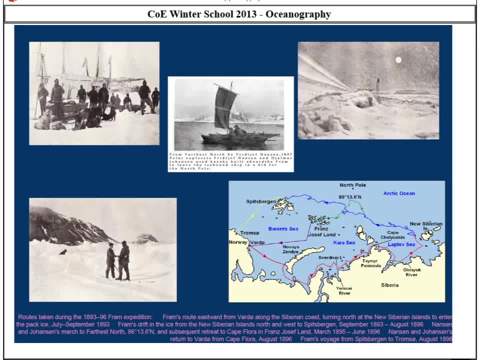 And kept them going. I think this is like a year and a half into it Where he started to go crazy and realized that they weren't going where they thought they were going to go, So the flow didn't follow the wind At this point in time. 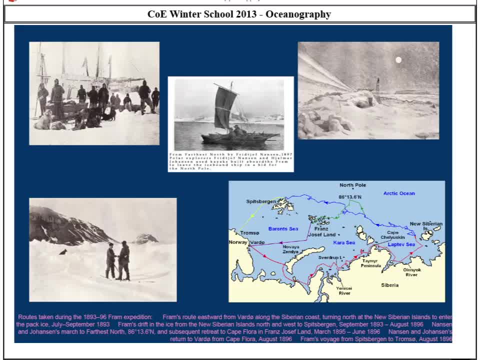 because he's insane, he mutinies, He's the captain and he bailed on his own ship. He hops overboard with his friend Olaf- Olaf Johannesson or something like that, And a bunch of dogs And he's like: 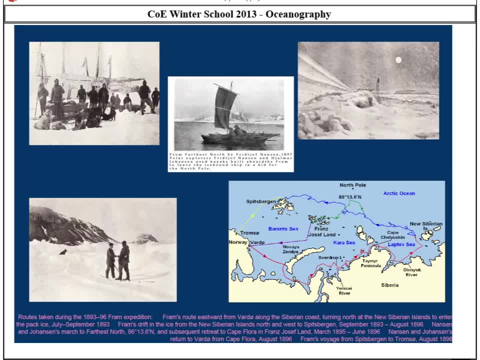 a bunch of dogs and some cross country skis And starts hiking And I think they spent like 6 months or something like that. They thought they'd try to get to the North Pole. This is, I mean. can you imagine? 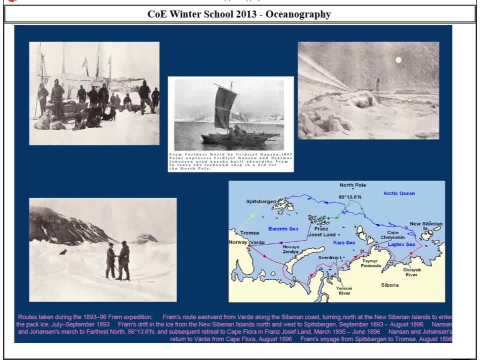 I don't know It's so nuts. Him and Olaf get all the way up here and they decide they're going to run out of food And they turn around and come back And they hike, hike, hike. They eat all of their dogs. 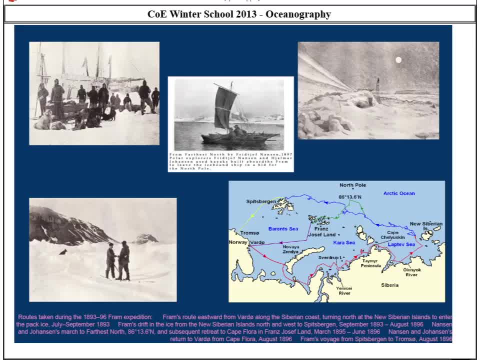 They build, they turn, like they also have these sleds that they then turn into sea kayaks. Anyway, they finally get to Franz Josef Land, where there's nobody. This is them in their sea kayaks. Yeah, And then they live. 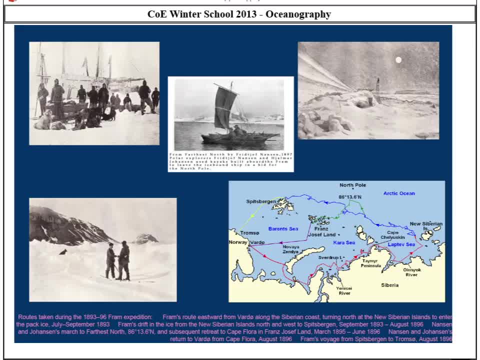 in this cave in the rock for like another 8 months and they spend a whole winter up there Eating like whales or- sorry, you know, seals and walruses and these things, And fending off polar bears because they're just covered. 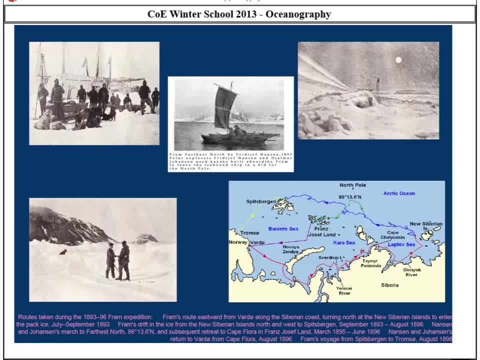 like dead things all around, Dead shotguns. Everything seems very hopeless. you know What are you going to do now? Lo and behold. I just think this is awesome: On June 17th, during a stop for repairs after the kayaks. 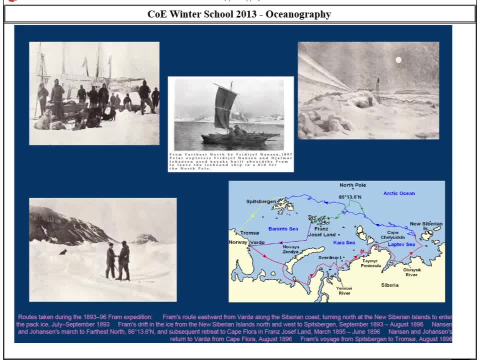 had been attacked by a walrus. Nansen thought he heard sounds of a dog barking and of voices. He went to investigate and a few minutes later saw the figure of a man approaching. It was the British Exchange Explorer, Frederick Jackson, who was leading. 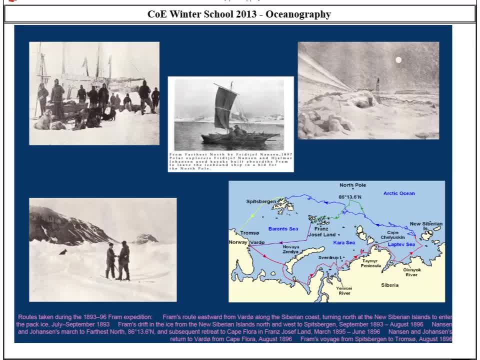 the expedition to Franz Josef Land and was camped at Cape Flora on the nearby North Brook Islands. You are Nansen, aren't you? And the receiver replied: yes, I am Nansen. So Nansen was soon picked up in the parrot. 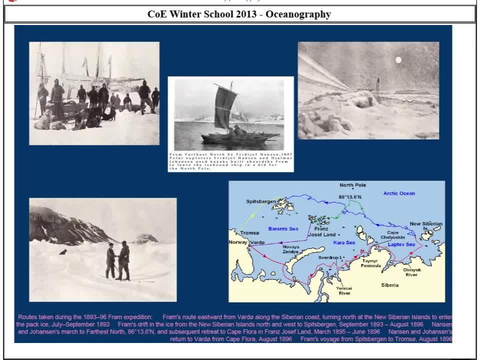 at Cape Flora. during the following stay with Cabrera in Florida, Nansen later wrote that he could still scarcely grasp the sudden change in Nansen's life. So he gets rescued here and he gets taken home. His bodies are still locked in the 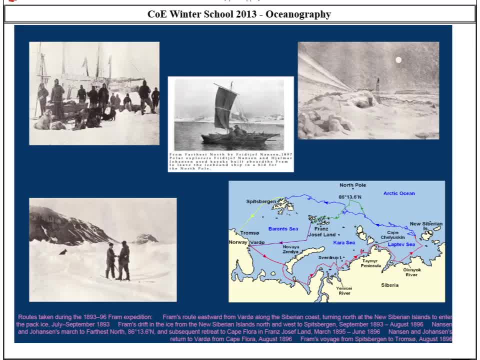 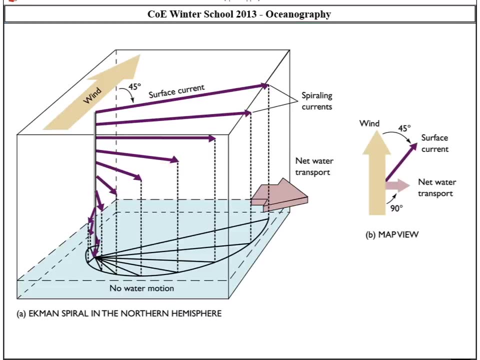 ice. He gets home before them. This is true. He did all sorts of other great things in his life, but some of the data that came out of that expedition was later processed by Wilford and his brother. Okay, 10 minutes, This is. 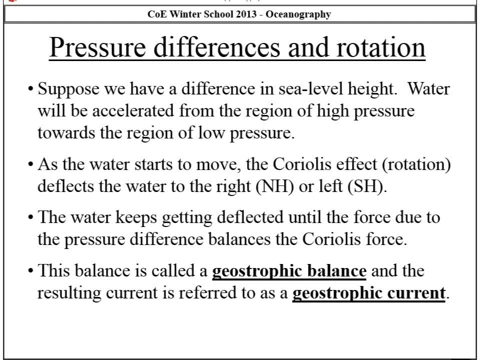 hopeless, Hopeless. Pressure and rotation. Pressure and rotation. Okay, there's pressure gradients driven by changes in sea surface height and differences in density. I'm feeling pressure gradients. I'm in the southern hemisphere, I'm moving in this direction. 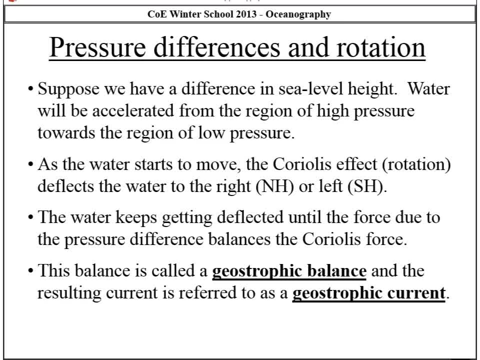 This is going to happen in the ocean. Where are these going to be the two most dominant forces? Pardon me Some topics, Yes, Sure, More importantly, where there's no friction. Okay, so these are the dominant forces. when you're. 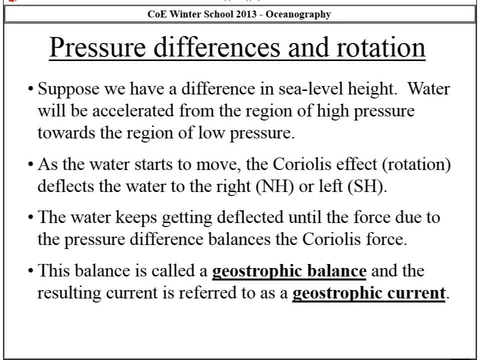 away from the surface or away from the pressure and rotation. This is called geostrophy. It's the same in the atmosphere When you go away from the boundary layer. it's just geostrophy. And so you feel pressure, gradient force, and there's no friction around it. You're moving this direction until the Coriolis. 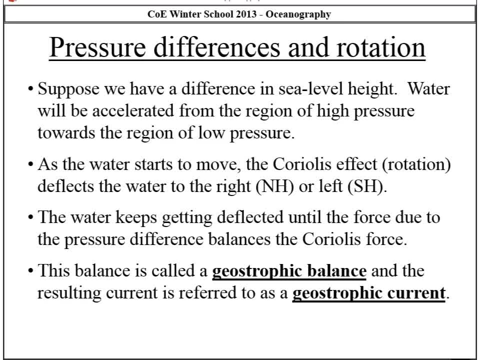 force kicks in and then you become a balance of the two forces. So if I'm in the southern hemisphere, my pressure gradient is this direction, my Coriolis force is this direction and I'm actually moving, at equilibrium, this direction which, let's face it, is totally weird. 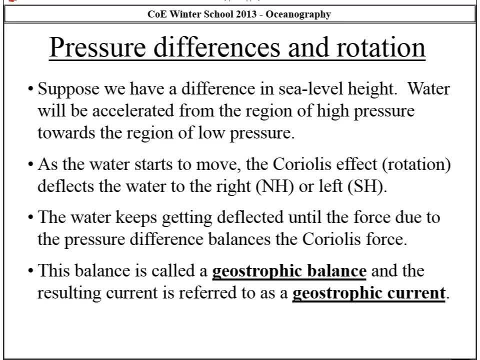 Okay If you do not move. you know ocean flows away from frictional boundaries, do not flow from high to low pressure, Unless you're right at the equator. Right It's going to be a balance between those two forces. So pressure gradient is this way: Coriolis force. 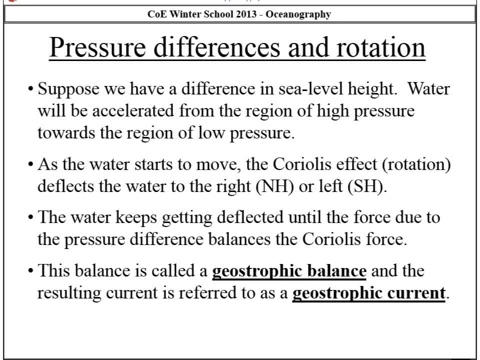 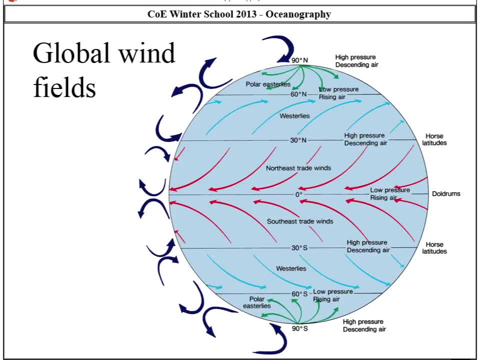 is this way, and the southern hemisphere is geostrophic, Flow does not flow from high to low pressure. Okay, Now, hopefully you have picked up a sheet of paper When you came in, did you? If you didn't, there should be one that someone can pass. 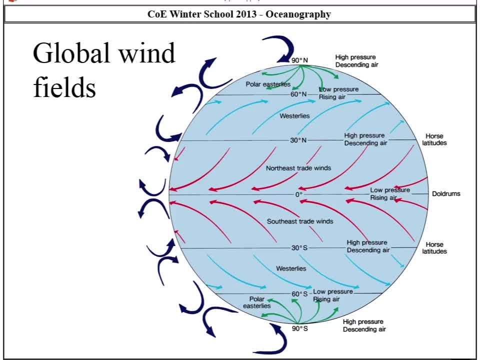 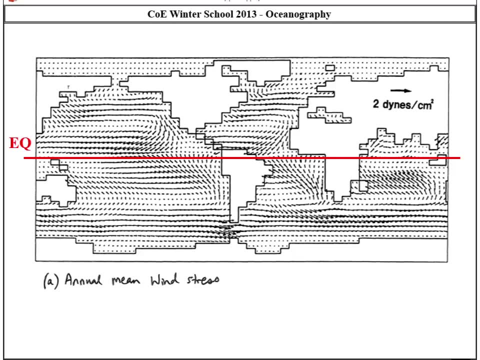 to you from this end. On this sheet of paper, it should look something like this. It's really crap. The arrows here are supposed to be the winds. Okay, So for let's do the tropical Pacific, the subtropical Pacific. The winds are blowing from east to west and they're 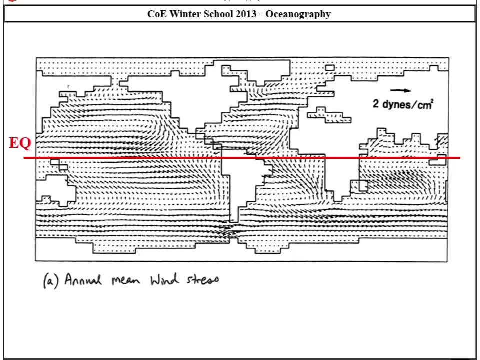 blowing from west here and from west to east here. That is your wind forcing. I would now like you, with your friends, feel free to talk- draw the direction of the Ekman transport. Winds are blowing this way and this way The Ekman transport is just the balance between 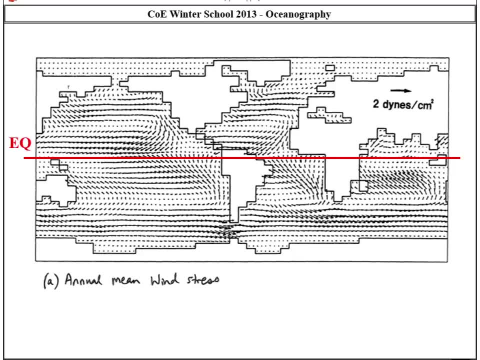 the wind stress and the Coriolis force, All right, And it's integrated over the whole upper Ekman layer and the net. Ekman transport is going to be 90 degrees to the right of the wind in the northern hemisphere. Have we got that? I'm sorry, I'm pushing you now. 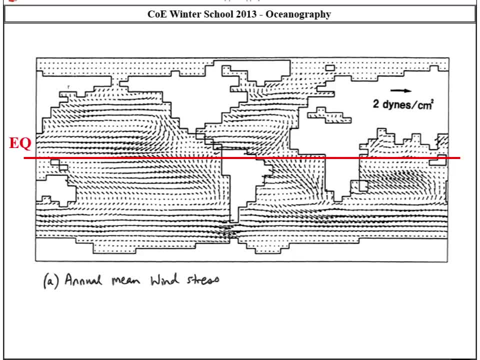 It should look the green arrow. they should look something like the Ekman transport. Does that make sense? You got this, Okay. Now what's going to happen? What's going to happen is all this water moving into the middle of this subtropical region. So, basically, you get this. 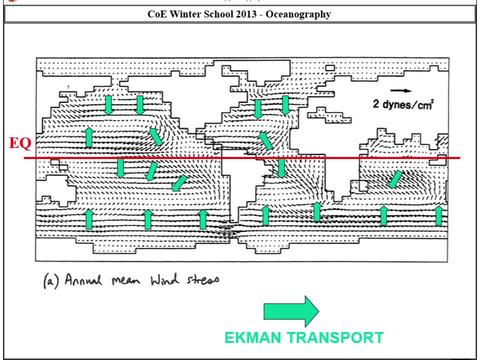 entire area is going to be in the expose When we do this. we're going to have a big plot. We're going to have rules. basically, We've got all these things here together. What is going to happen to the sea surface height there? 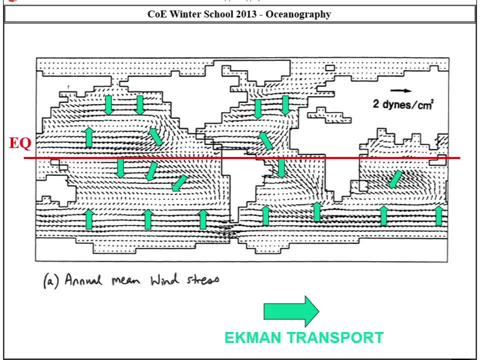 Higher or lower? Raise your hands Higher- It's going higher, It's going higher. We now have an elevated sea surface height in this region. Now imagine you are a little parcel of water down below this frictional wind layer. You are now feeling a region of high pressure. 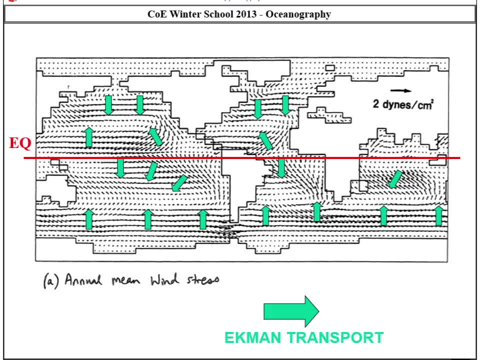 Draw a big H here, Put a circle around it. This is now your pressure gradient. I would now like you to draw the direction of the geostrophic flow at depth. Does that make sense? Feel free to talk amongst yourselves. Here we go. I'm not here. 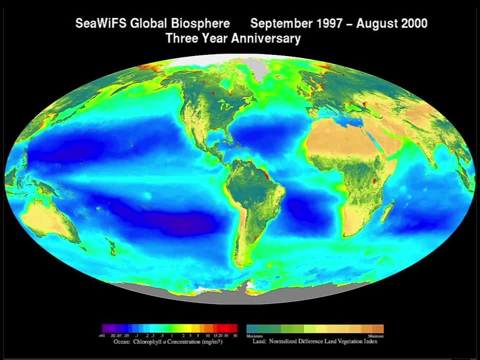 You think, yep, Okay, in here, No, no, no, sorry. In the other areas, the lighter colors- Yeah, the lighter colors is where you have upwelling. Yeah, for sure. Why does upwelling lead to primary production? 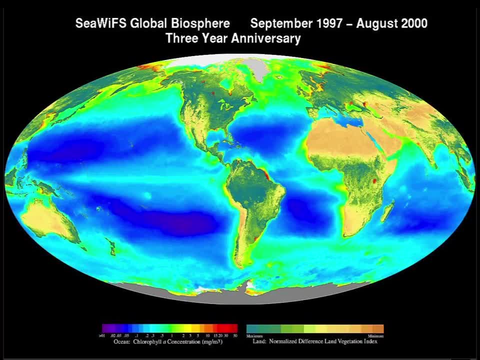 Yeah, so the primary production of these? phytoplankton or whatever? right, they need light and nutrients, So they've got to be near the surface and they need nutrient sources If they run out of nutrients, if there's no resupply of nutrients. 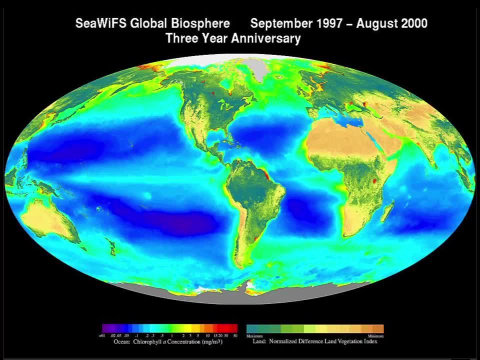 then they die off. So phytoplankton eat, then they poo or die, fall to the bottom. So somebody's got to get those nutrients back up from death. So where there's regions like here, you have a lot of what we would call upwelling. 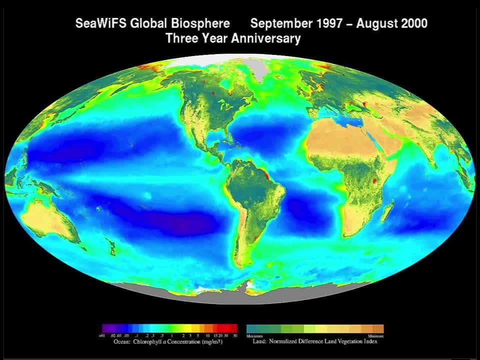 Or the hot spots would be near rivers, where it's bringing nutrients from the rivers. Okay, why is there? let's deal with this spot here, because it's easier for people. Why is this spot? why doesn't it have nutrients? We built this high pressure right by the Ekman transport in those regions. 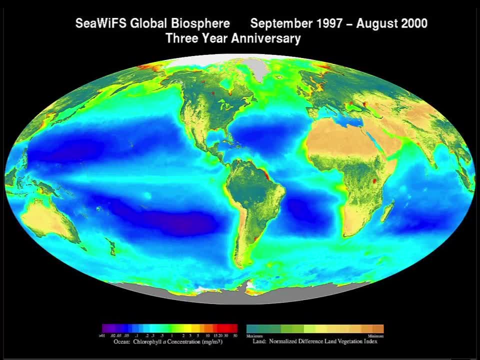 Does that make sense? So the winds here are blowing this direction and this direction. The Ekman transport at the surface is into the middle of this region, piling up sea surface height. What is that going to do to the ocean flow there? 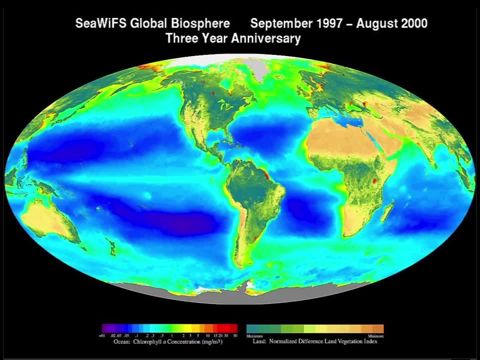 The vertical ocean flow. Yeah, if you make a big bulge of water there, it's got to go somewhere And it's going to lead to some gentle downwelling. This isn't like convection, you know, making North Atlantic deep water and stuff. 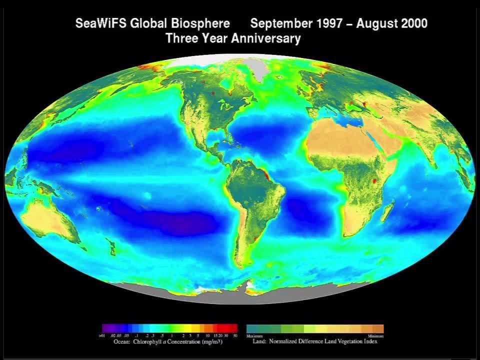 This isn't you know, this is going. this is happening over the first maybe 500 meters or so, But it is general trend for downwelling in those regions. Okay, And so the fishies that are trying to live here. it's very hard for them to get nutrient resupply. 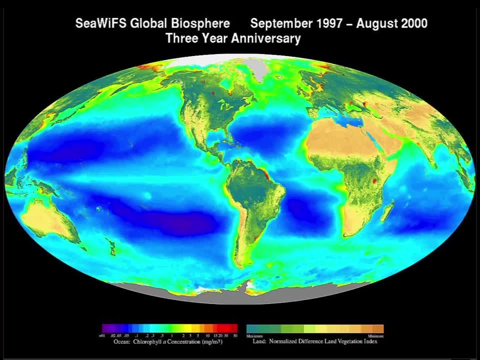 Okay, Here there is a big nutrient resupply. What's happening here? Okay, Upwelling. Can someone tell me why there's going to be upwelling here? Yeah, Pardon me. Yeah, you've got a lower sea surface. 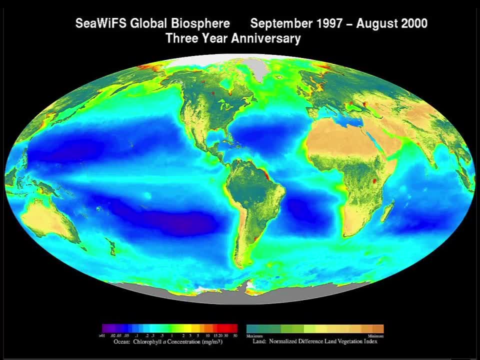 You've got a lower sea surface. So what's causing the lower sea surface? Yeah, Yeah, exactly. So in this region here, the winds are blowing in this direction, right, If you're on the southern side of the equator. 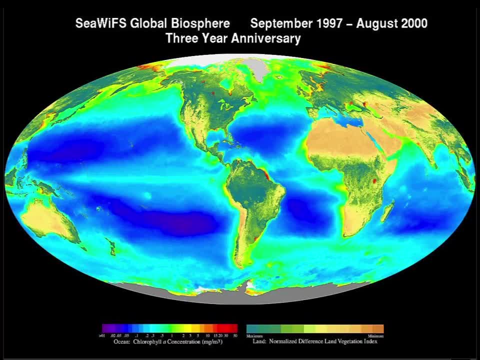 where's the ecumen transport? So away from the equator. If you're on the northern side of the equator, the ecumen transport is to the north, leading to upwelling in this region. I have to stop. I'm sorry. 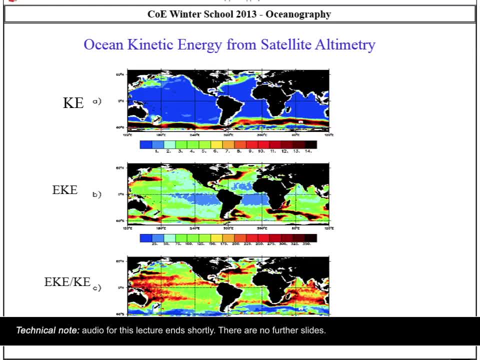 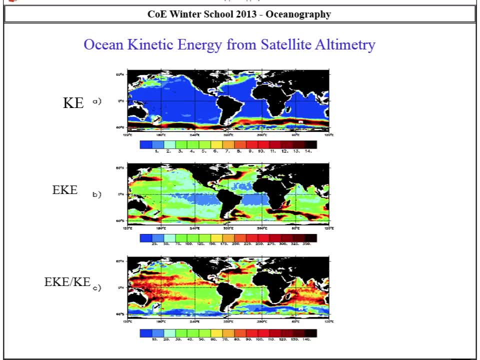 I will just point out one last thing, because this needs to be said. Everything we've been talking about here is what the mean ocean states. These mean currents. This is something that was done by Carl Worms, showing the kinetic energy of the ocean. 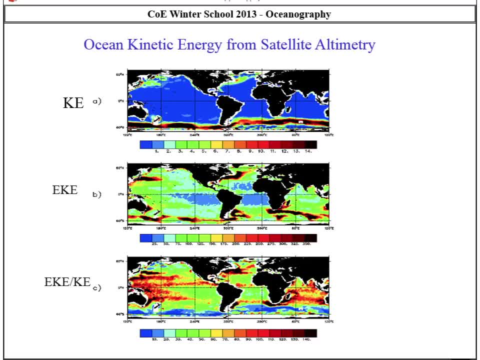 Okay, This is the mean kinetic energy of the ocean. The red spots mean it's high kinetic energy. The blue spots mean it's low. But notice the scale: It goes from 1 to 14.. Okay, This is the energy in your mean currents. 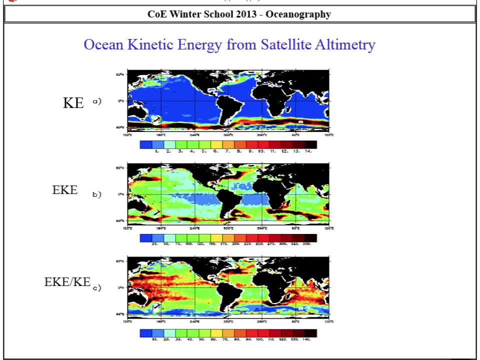 This is your energy in the eddies, or the transient motions. Okay, The variability away from the mean. Okay, Notice the color scale goes from 25 to 350.. 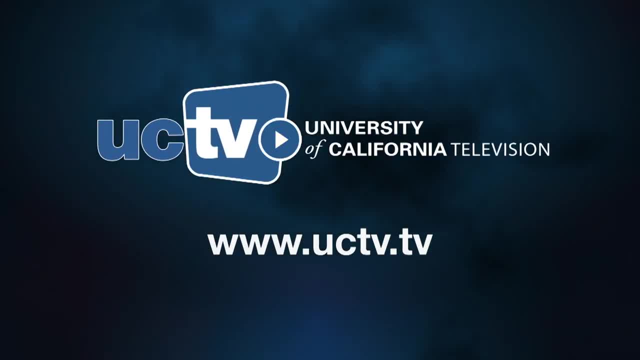 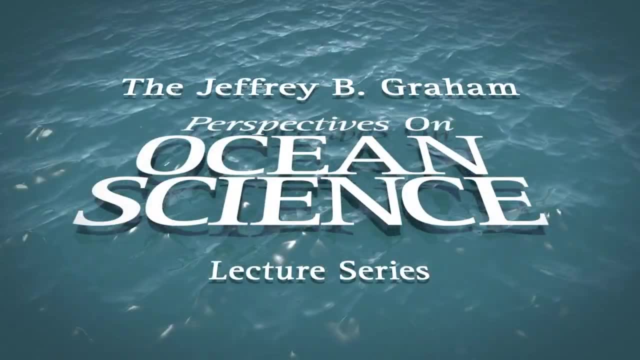 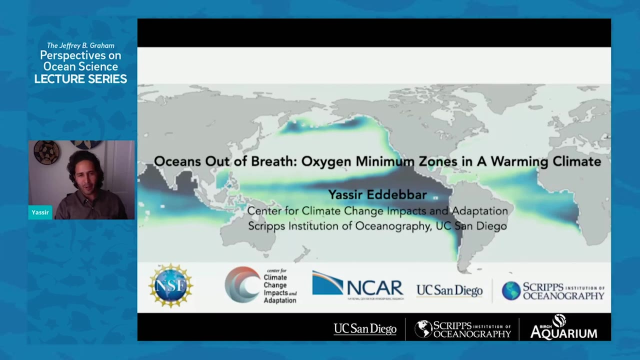 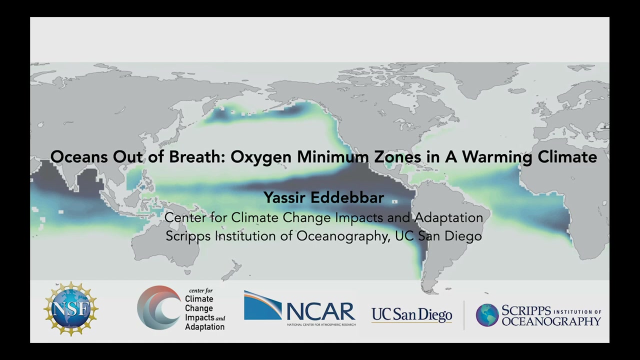 Oxygen is really fascinating and it's really special for a variety of reasons. One of the main reasons we study it is that it's really important for life in the ocean. Without oxygen, there's simply no life in the ocean, Just like there's no life on land without oxygen.